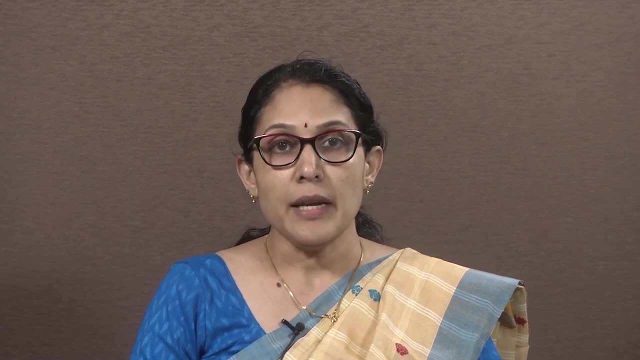 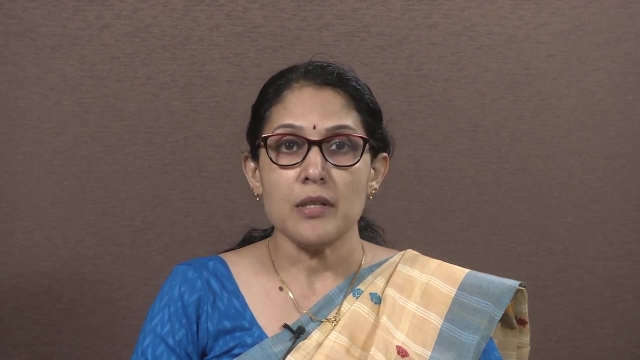 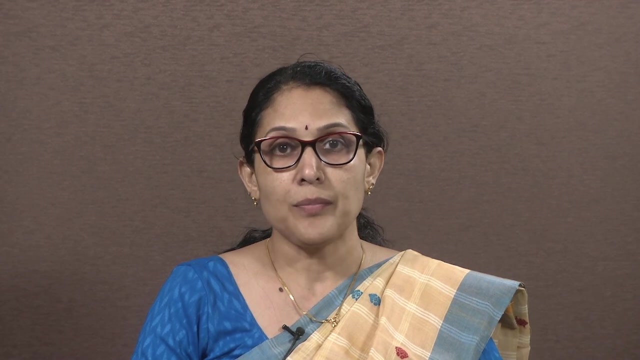 product of velocity and cross sectional area. So in this case we are considering the average velocity. So how to calculate average velocity? that also we have seen Today. let us move on to the topic of Representation of Streamflow. Representation of streamflow. 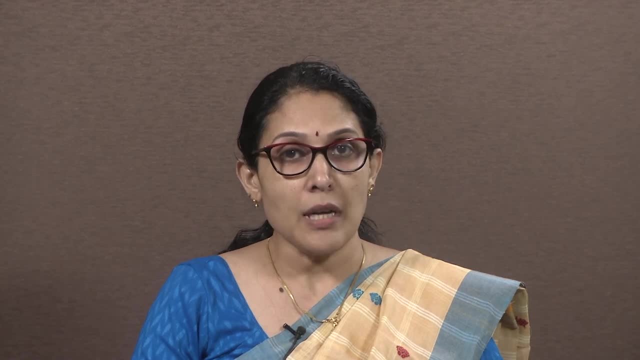 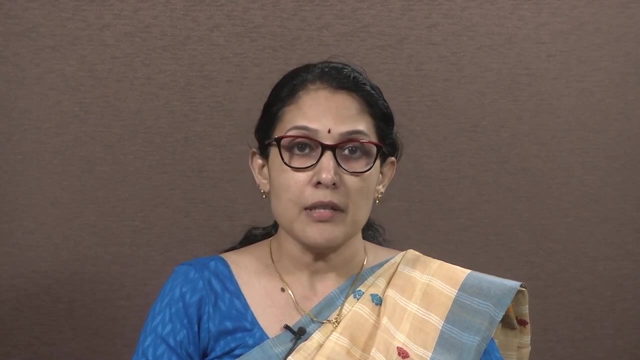 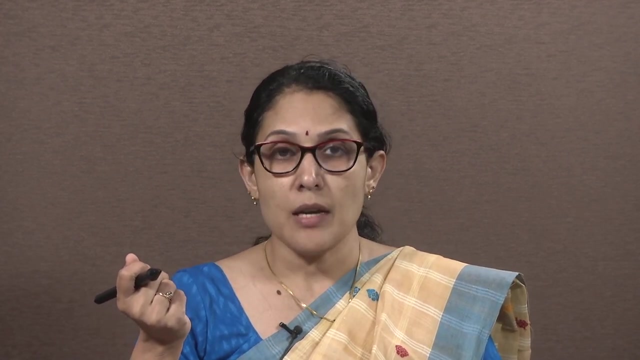 means the measured values for different time intervals are there with us, and how to represent that data in a graph. that is what we are going to see in today's lecture. The representation of discharge versus time is termed as stream flow hydrograph. We already know. 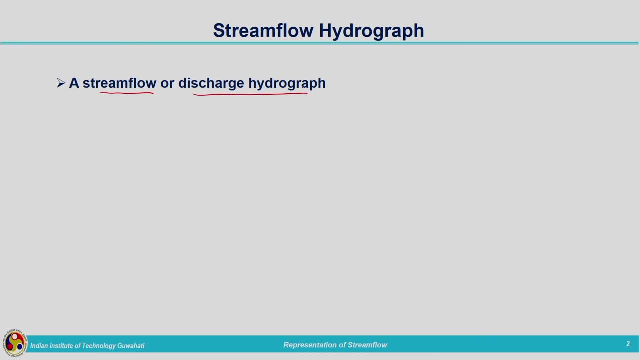 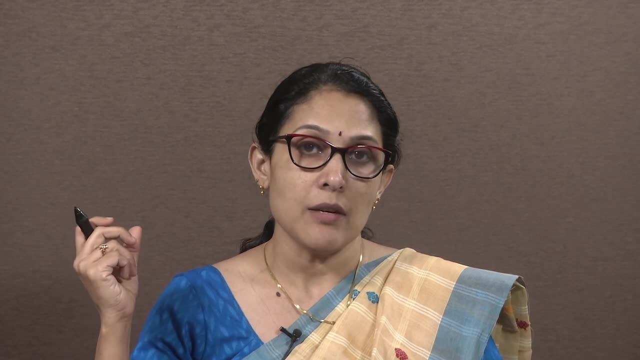 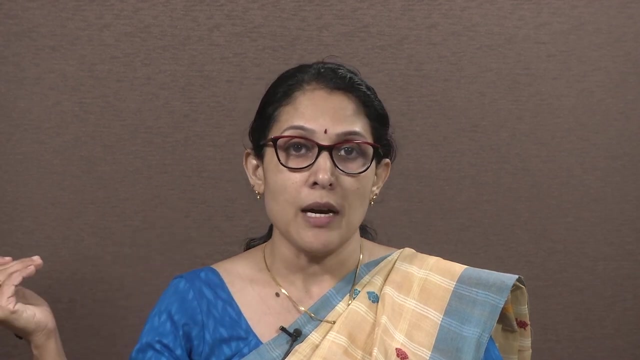 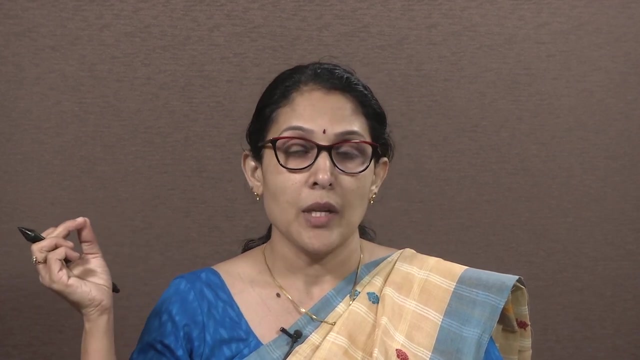 how to calculate the stream flow at a particular gauging station. Water levels and the corresponding velocities at a particular gauging station will be measured. based on that we will be calculating the stream flow. If it is continuously observed over time, then we can get the stream flow details corresponding to all the time. So this: 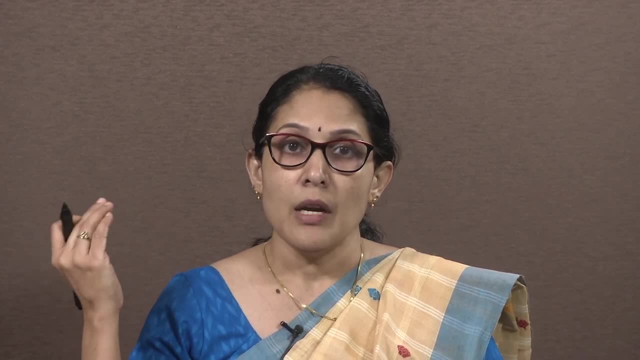 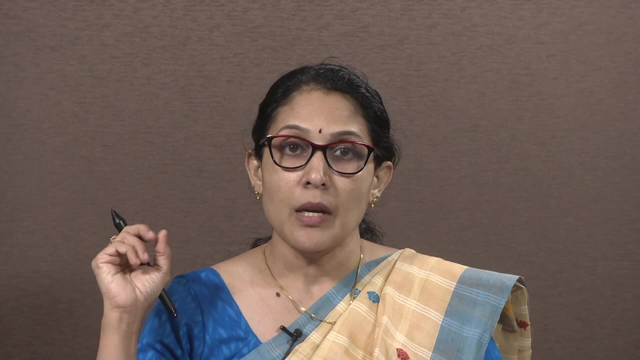 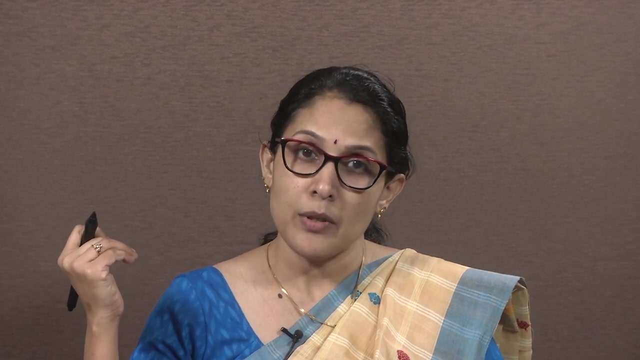 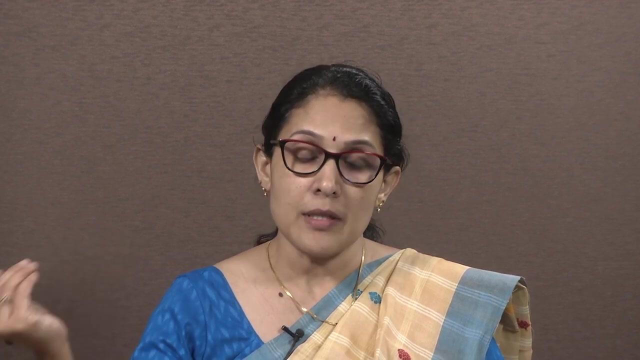 is similar to that of a rainfall hydrograph. In the case of rainfall hydrograph, we are plotting rainfall intensity with respect to time. It is a discrete curve. but when we talk about stream flow hydrograph, this is also plotted with respect to time, to flow rate with respect to time, but this is a continuous curve. That is the graph showing. 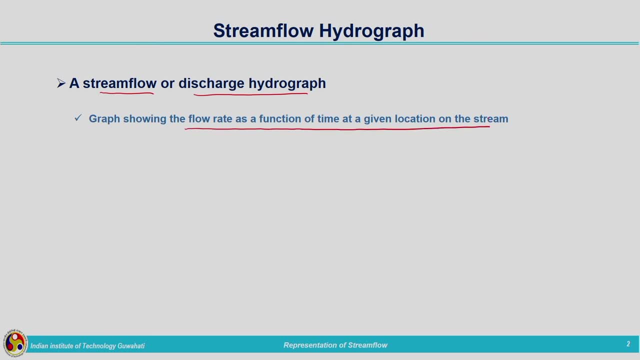 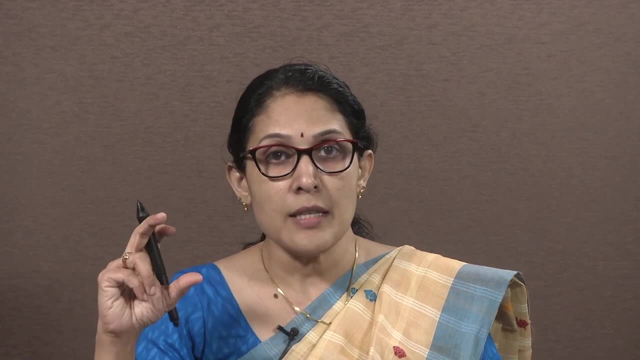 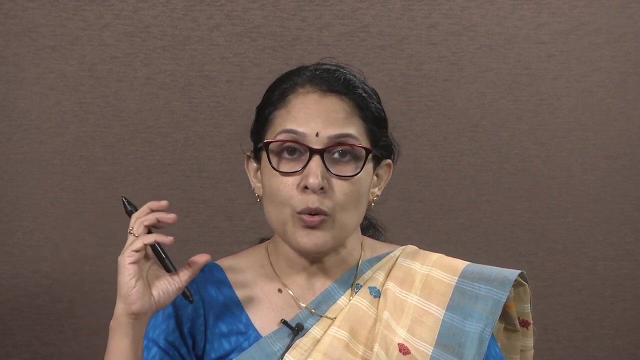 the flow rate as a function of time at a given location on a stream. that is our stream flow hydrograph. So if you are plotting the water level or the stage at a particular station with respect to time, then it is termed as stage hydrograph. So usually for hydrologic analysis we will be 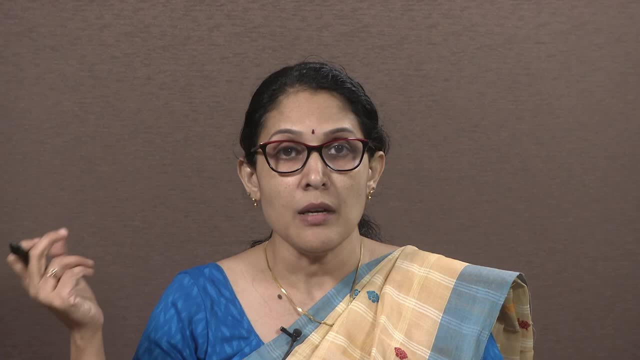 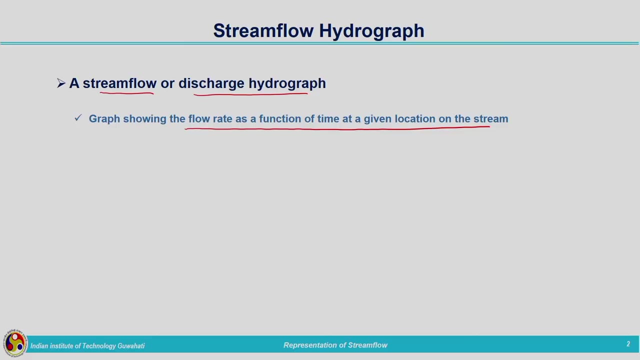 making use of the stream flow hydrograph, in which the stream flow or the discharge at a gauging station is plotted with respect to time. Different ways of representing stream flow hydrograph. one is annual hydrograph. second one is term hydrograph. From the name: 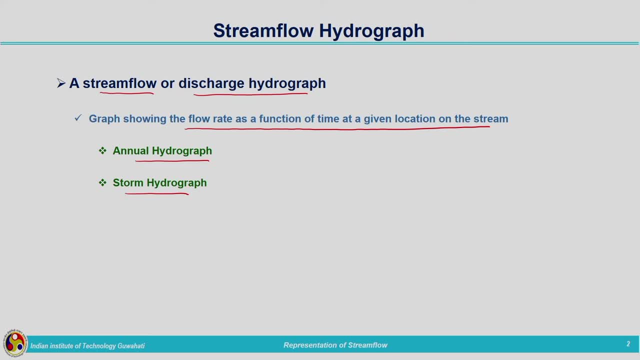 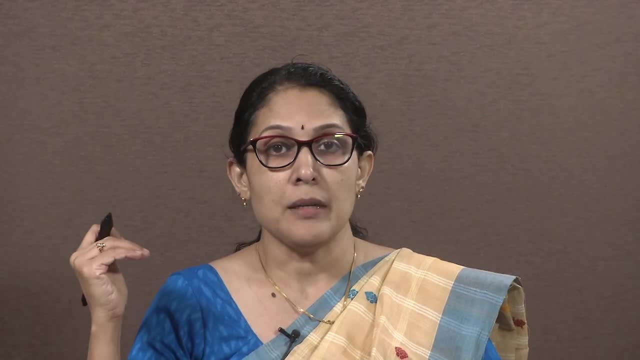 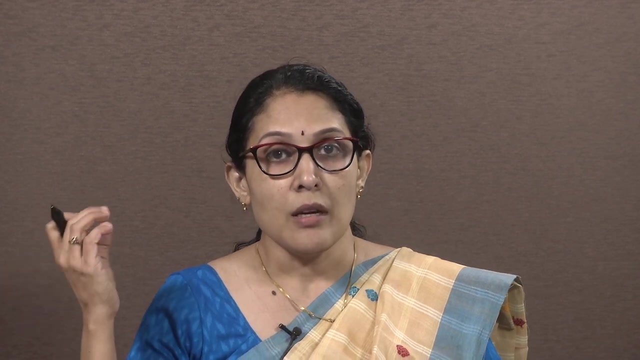 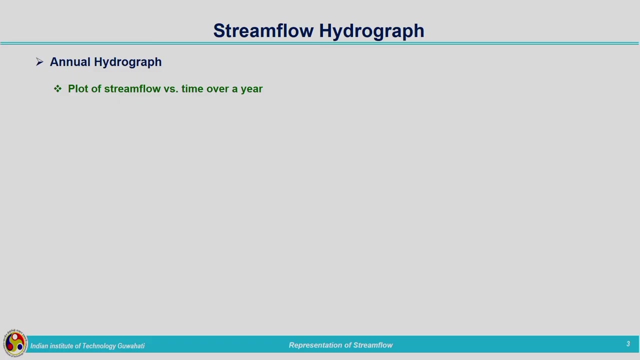 itself. it is clear that annual hydrograph will be representing the flow data for the entire yourself year, and storm hydrograph is the one which is representing the stream flow at the gauging station corresponding to a particular storm. let us see one by one. first one is the annual. 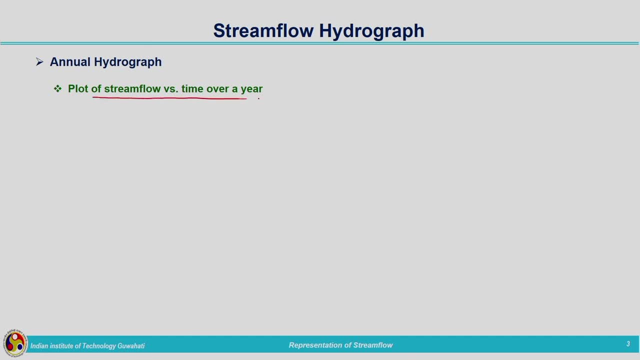 hydrograph. the plot of stream flow versus time for a complete year is the annual hydrograph. so if you are measuring the stream flow for the entire year and it is plotting as a hydrograph, that is what is termed as the annual hydrograph. this shows the long term balance of precipitation. 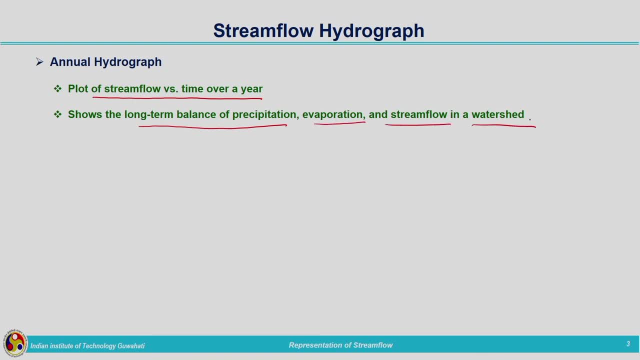 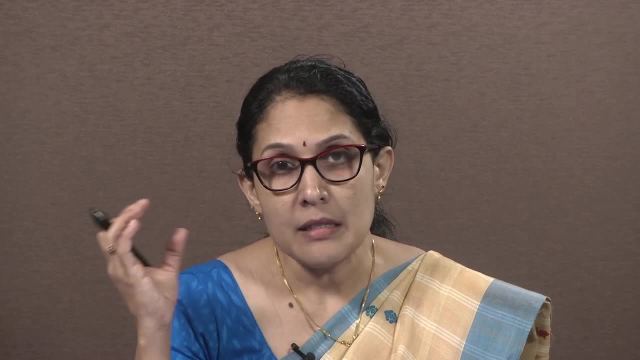 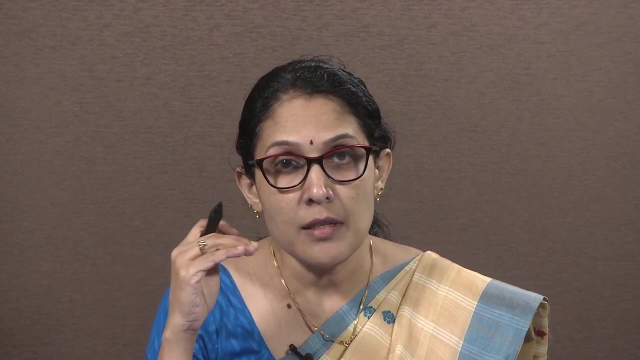 evaporation and stream flow in a watershed. from the annual hydrograph we can understand how the water balance is taking place, how the stream flow variation is taking place in a catchment, because if you are considering the data corresponding to the entire year, in certain months we will 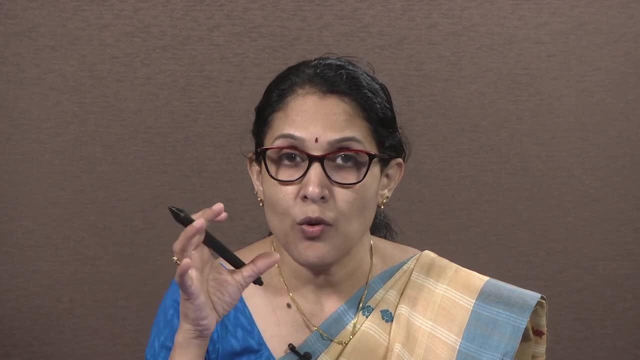 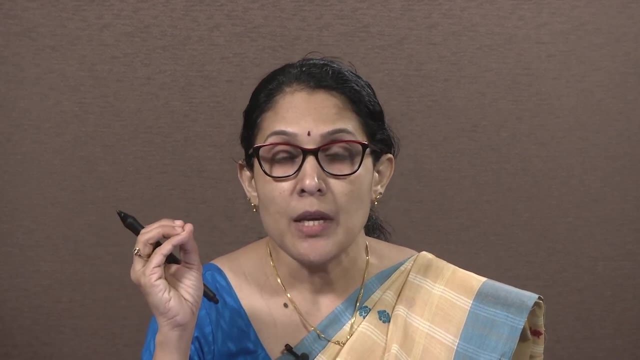 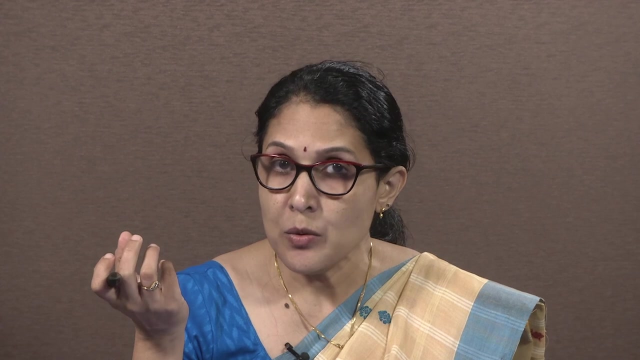 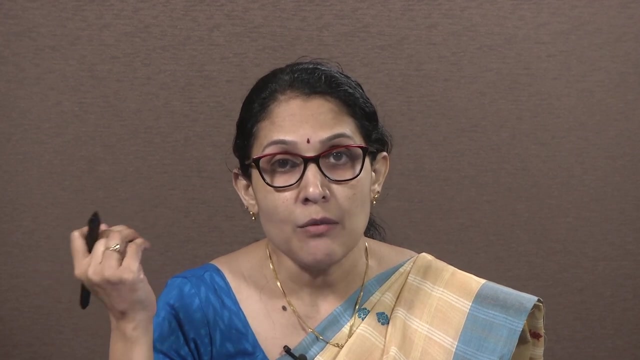 be having rainfall. during some other months we won't be experiencing any rainfall. so the representation of stream flow we know already. stream flow is consisting of surface runoff, interflow and also base flow. during the monsoon season only the contribution from the rainfall and interflow will be coming. rest of the season we will be getting water in the rivers by means of. 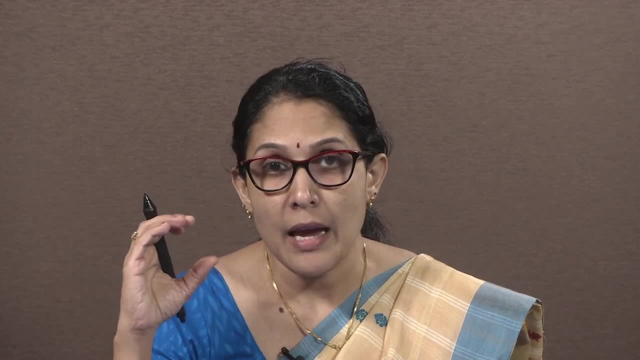 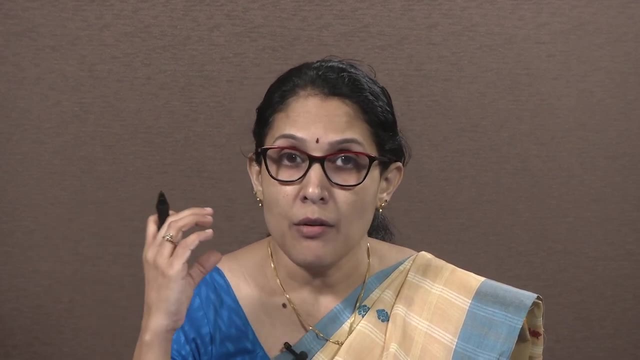 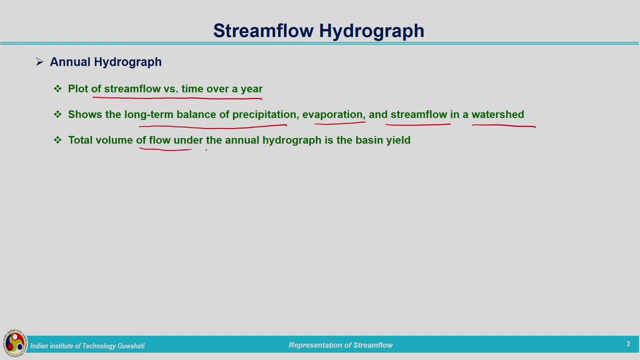 base flow. so if we are analyzing the annual hydrograph, we will get a clear picture of the contribution of water to the stream from surface runoff interflow and also base flow, and the total volume of flow under the annual hydrograph is the basin yield. so whenever a catchment watershed 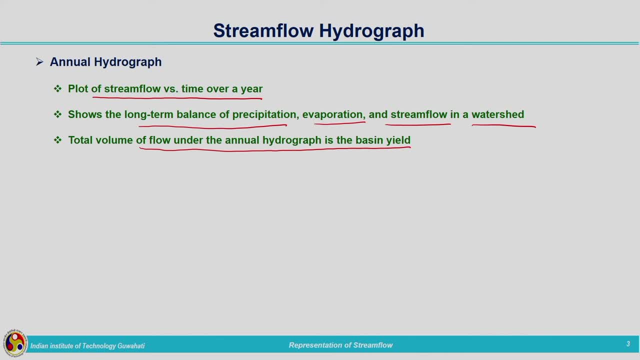 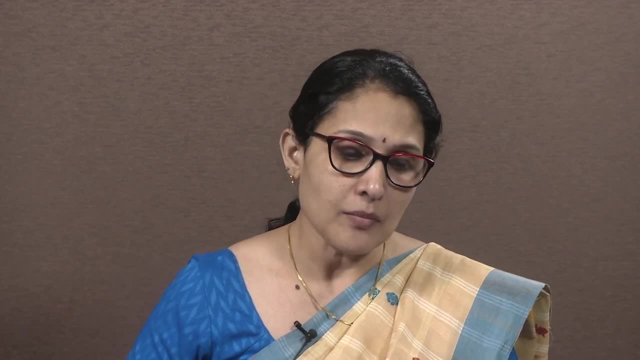 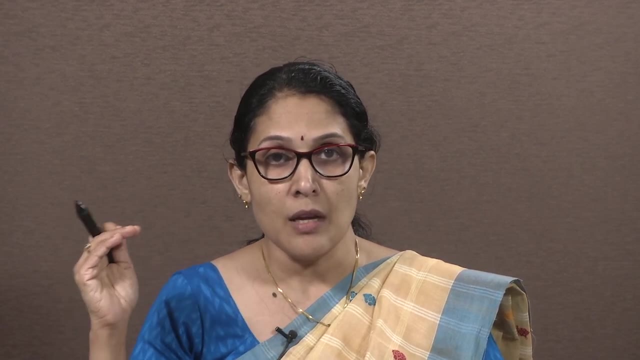 or basin is concerned, the total stream flow which is observed there, at the outlet point, is termed as the basin yield. in yield, that is the total volume of flow under annual hydrograph. Annual hydrograph is representing the flow variation or stream flow record against time. 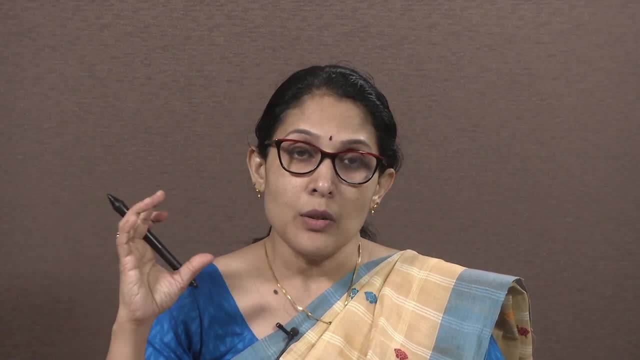 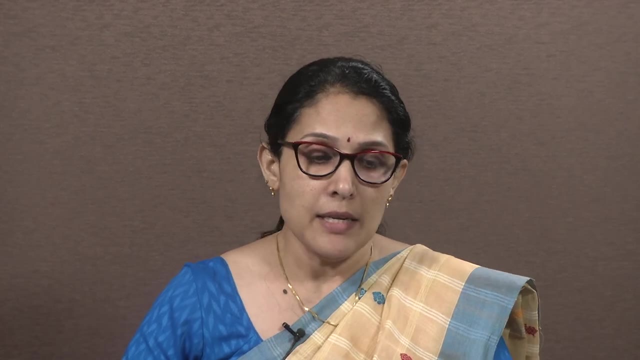 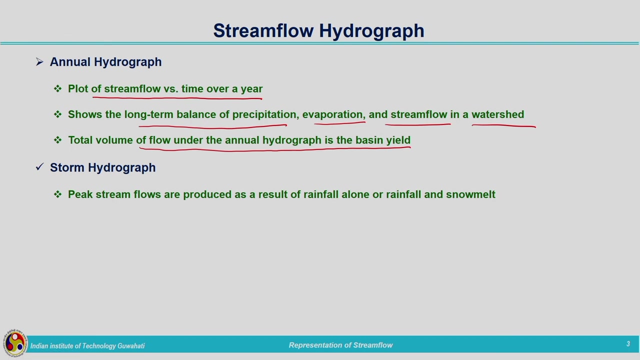 in a single graph for the entire year. So the total volume of flow under the annual hydrograph is termed as the base in yield. Second one is the storm hydrograph. This is the storm hydrograph is the one which represents the stream flow versus time during. 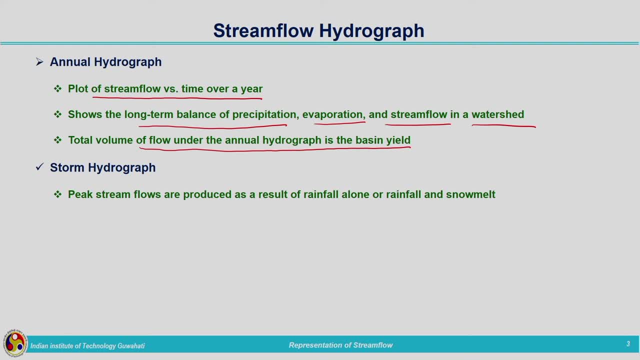 the time of a particular storm or rainfall, So peak stream flows are produced as a result of rainfall alone or rainfall and snowmelt. Some of the catchments will be getting water due to rainfall and snowmelt, and some other catchments will be experiencing runoff based on rainfall. 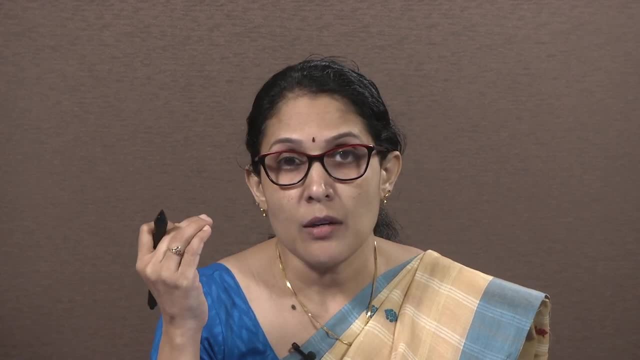 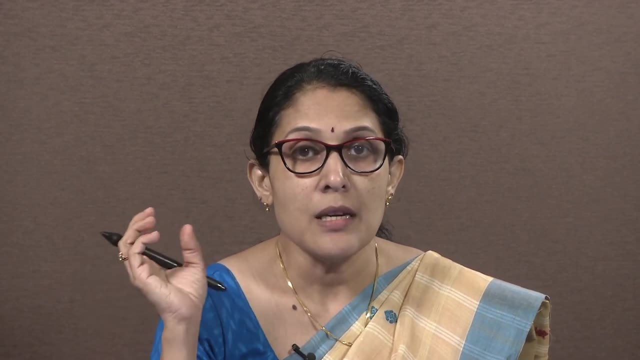 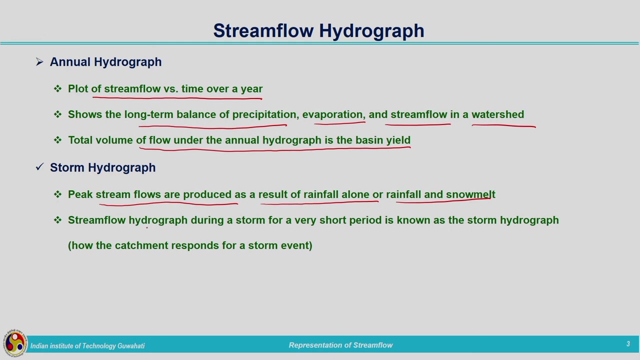 So the peak stream flows are observed during the time of rainfall and in the catchments where the snowmelt is also taking place. it is a combination of rainfall and also snowmelt, So stream flow hydrograph during a storm for a very short period is termed as storm hydrograph. 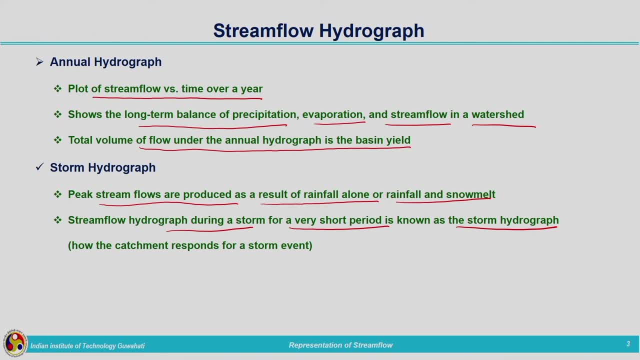 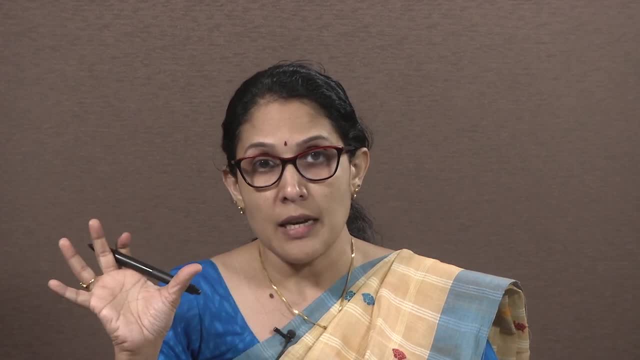 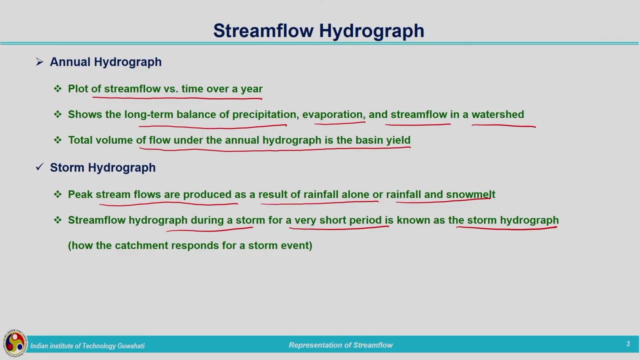 That is, in the annual hydrograph we are plotting the stream flow versus time for the entire year. But in the case of storm hydrograph we are not considering the entire year. we are considering the period corresponding to that particular storm or snowmelt is taking place. 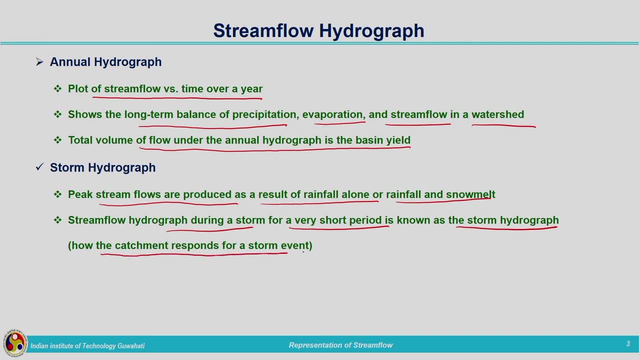 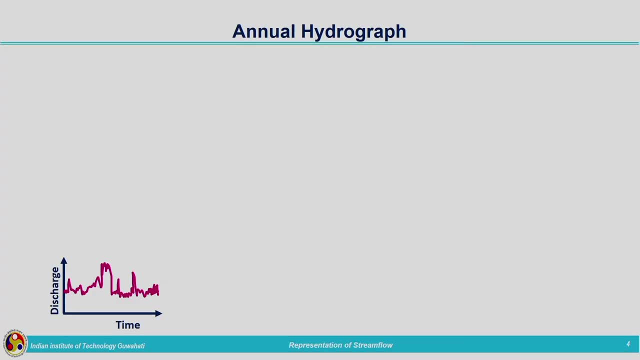 That is, it is the response of catchment corresponding to a storm event. Now we can see different types of annual hydrographs. when we plot, along the x axis, we are having time- this is corresponding to the entire year- and along the y axis, we are having the stream. 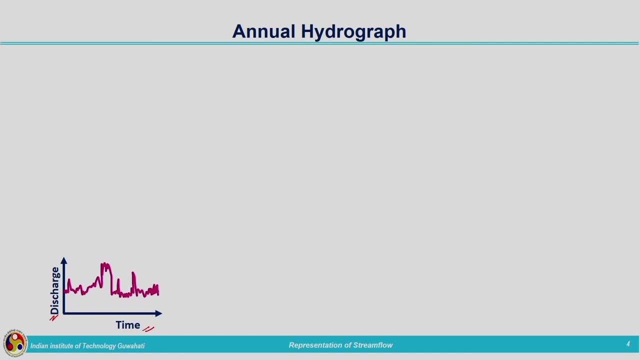 flow. So in the case of storm hydrograph we are considering the entire year and along the y axis we are considering the discharge in meter cube per second. So here you can observe that these lines are representing the discharge variation or the stream flow variation in a particular catchment or basin. 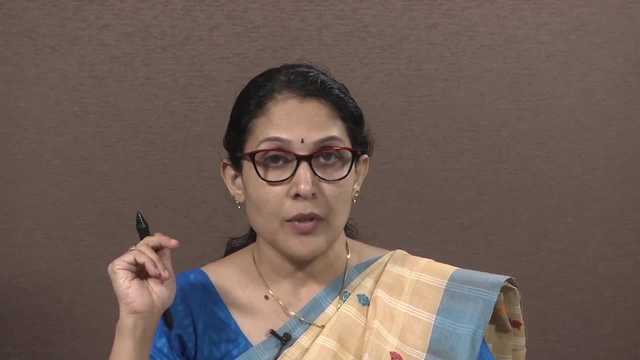 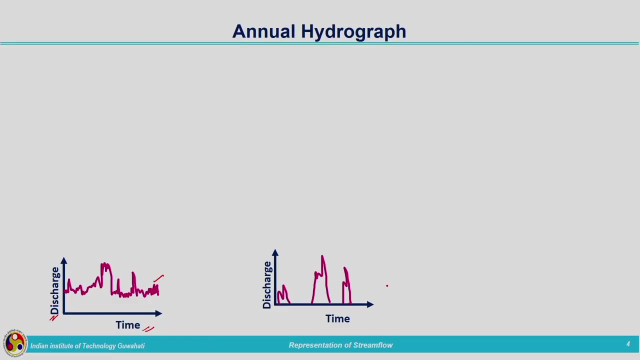 So this is having. when you observe the curve, you can see for the entire period of one year. it is displaying the flow or discharge, And the second one is for the schools year, in which we are having in extreme flow at certain periods only. This is for a time, is for the entire year and you can observe that the peaks are the. 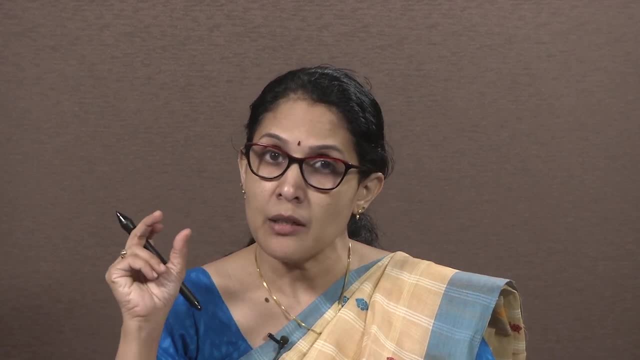 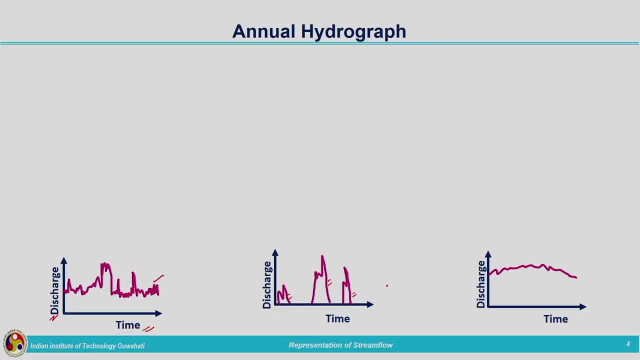 or the flow details are the corresponding to certain period of year, not for the entire year, And there is third kind of annual hydrograph. here you can see, from beginning to end we are happiness stream flow and there is not much variation taking place in the stream flow value From the beginning to end. 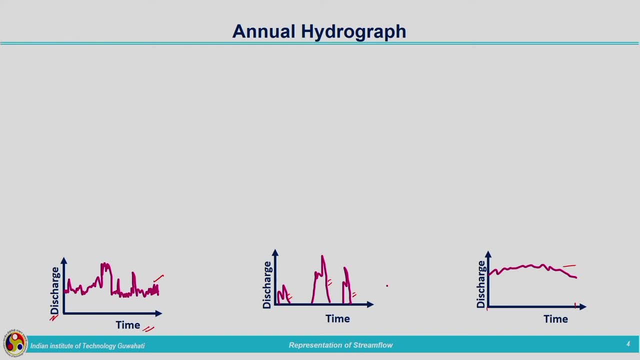 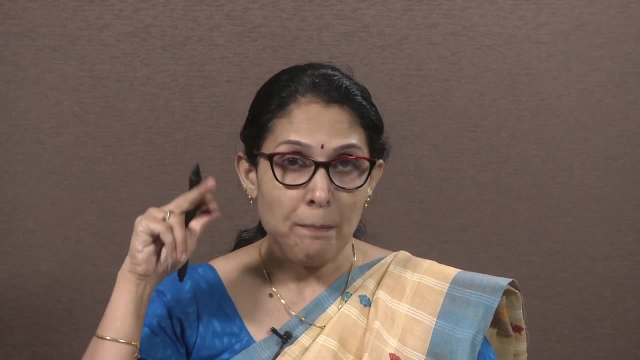 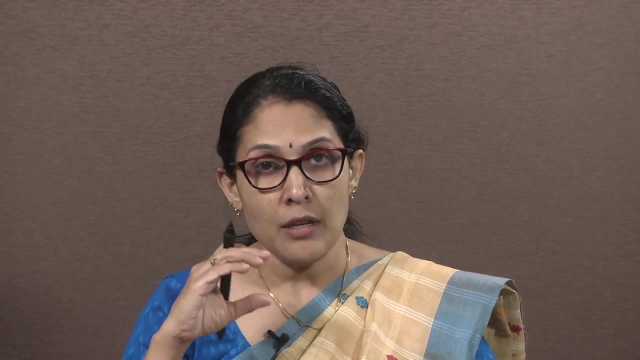 it is approximately of the same value. Slight variation is there, but still more or less it is following a similar trend. There is no peaks coming into picture. So you can compare all the three graphs. In the first one we are having flow for the entire period of year, but there are so. 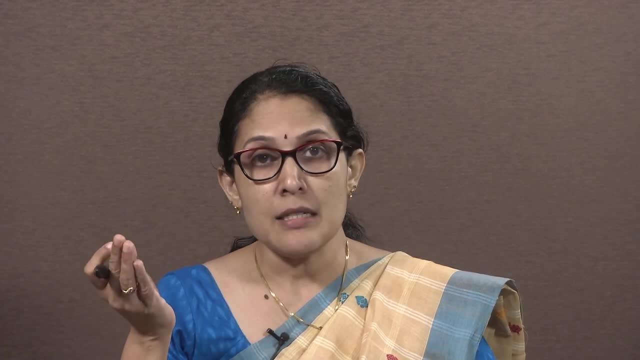 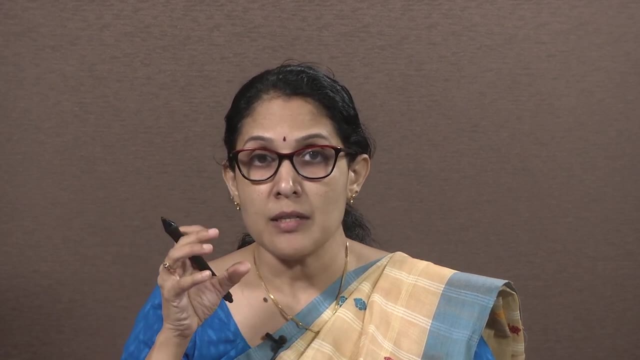 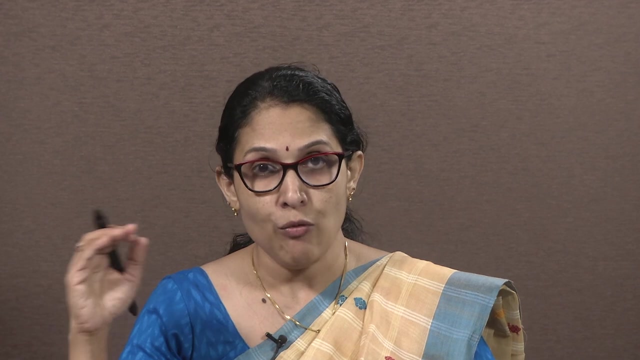 many spikes coming over the graph And in the second graph, certain periods only. we are having stream flow. In between we are not having any stream flow records And in the case of third one, for the entire one year we are having water or flow in the stream, but there is not much variation. 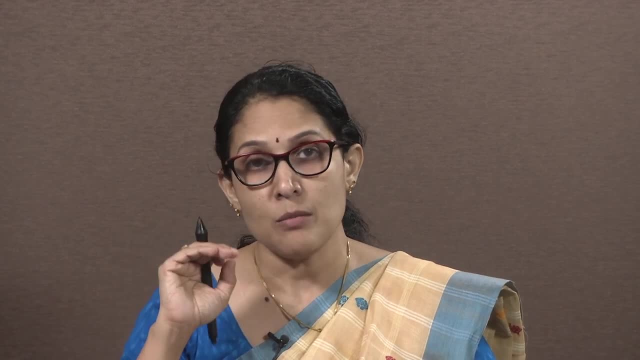 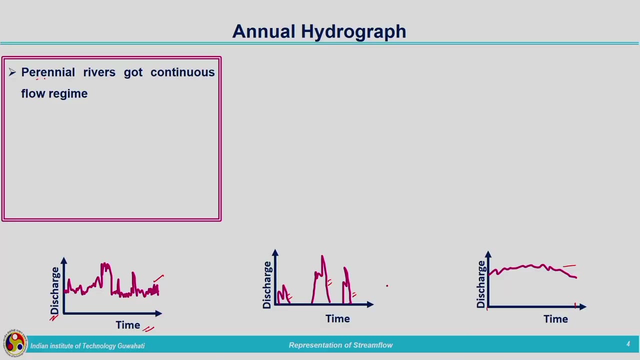 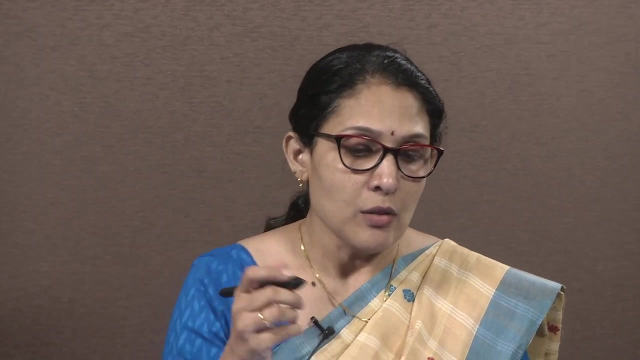 in the representation of the stream flow values. It is more or less a steady value. So the first one is characteristic: We are responding to the stream flow hydrograph from the perennial rivers. Perennial rivers means the rivers which are having water all throughout the year, So it got continuous flow regime. 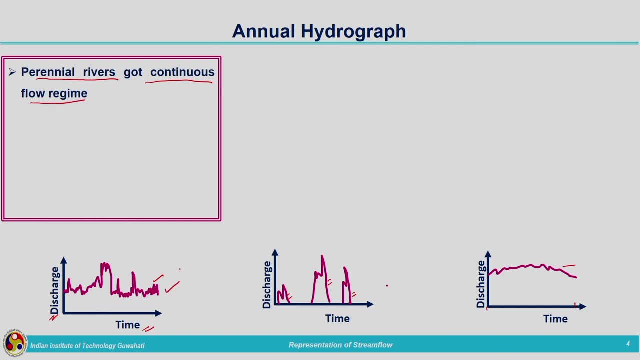 That is why we are having a stream flow representation like this. For the entire period, we are having the flow within the river And most of the basin yield usually comes from base flow. In this case, most of the basin yield is coming from base flow. 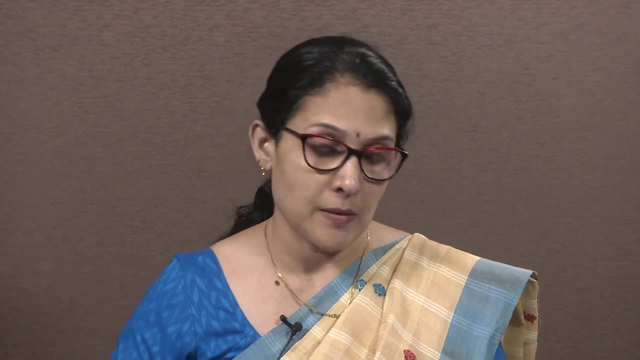 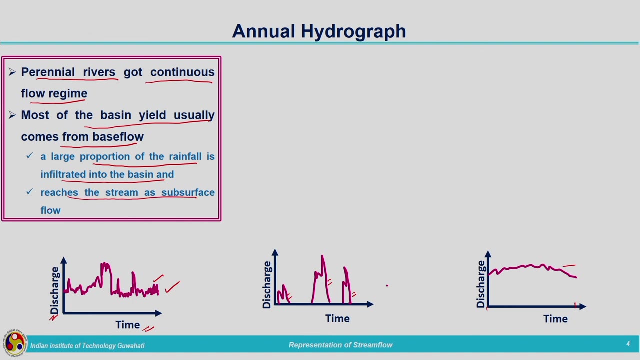 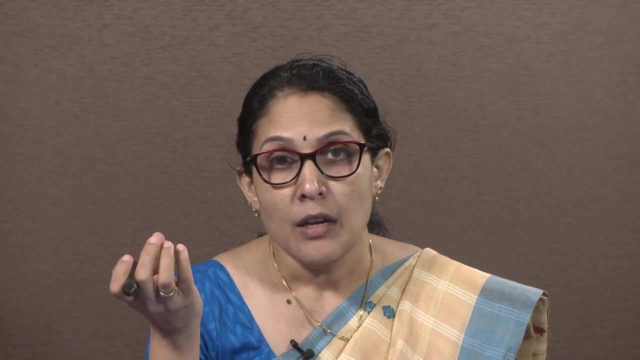 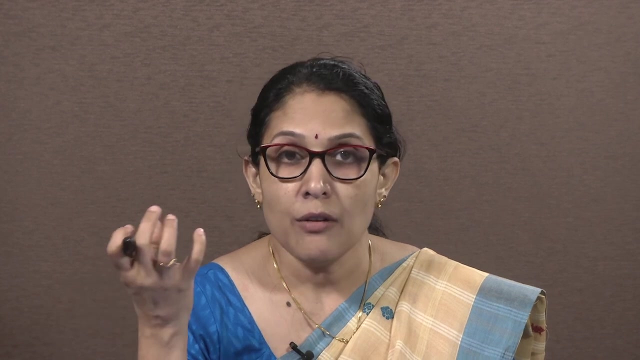 but the spikes are represented by the storms. A large portion of the rainfall is infiltrated into the basin and reaches the stream as a subsurface flow. So for the entire period of year if we are getting stream flow means even though there is no rainfall, water is contributed towards the stream as stream flow. So definitely it should. 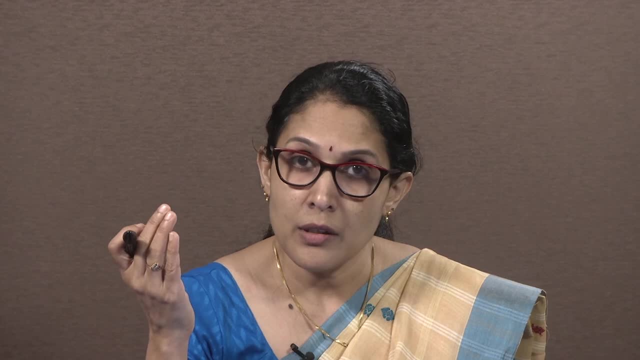 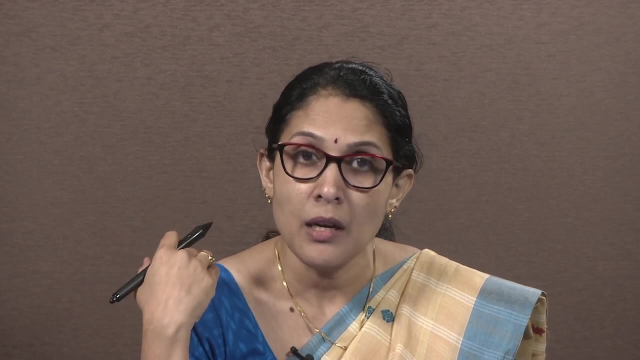 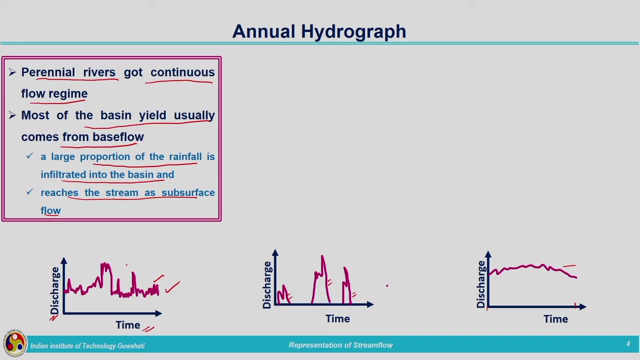 come from the base flow, So majority of the water during the time of storm will be getting infiltrated into the ground and it will be meeting the groundwater table and water will be flowing towards the stream as in the form of base flow. That is the reason why we are experiencing flow. 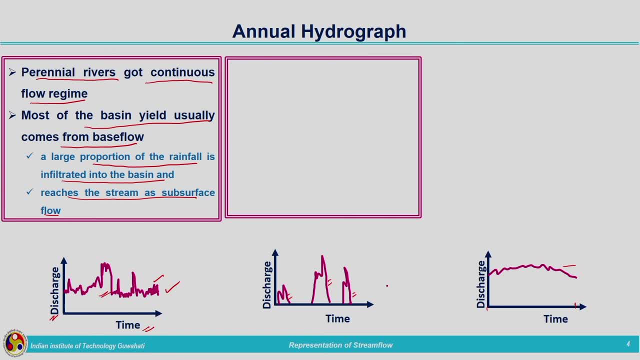 all throughout the year. In the second one, we are experiencing stream flow during certain periods only. These are corresponding to ephemeral rivers which are having periods with no water when the river is dry. You might have observed certain rivers are dry during non-monsoon season, So the river will 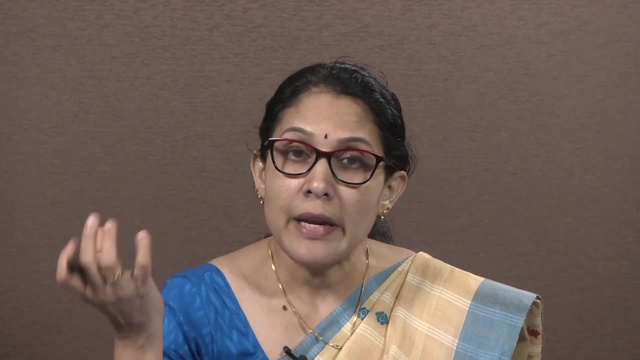 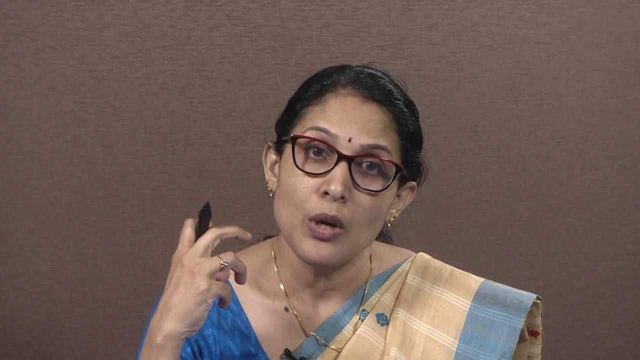 be flowing only during the time of rainy season. That is, most of the stream flow which is coming to those type of rivers is due to rainfall. So in such regions the infiltration component becomes very important. So in such regions, the infiltration component becomes very important. 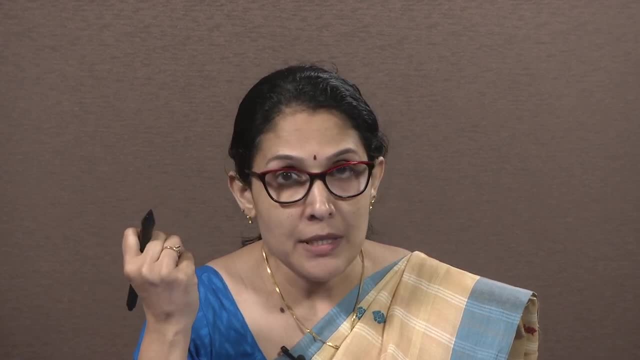 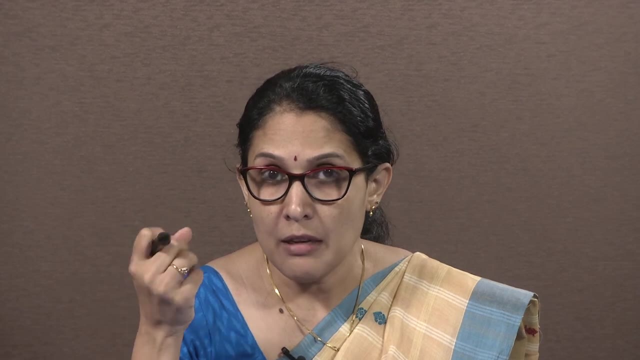 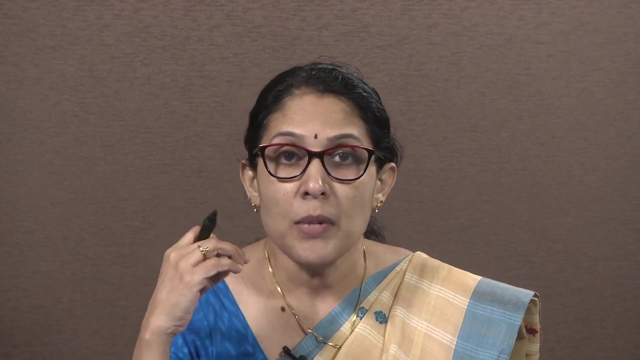 So in such regions the infiltration component becomes very important. So in such regions the infiltration will be less and whatever form precipitation is occurring, majority is coming as runoff and meeting the stream. Since the infiltration component is less, the contribution from storm to the ground water is very less. because of that, the 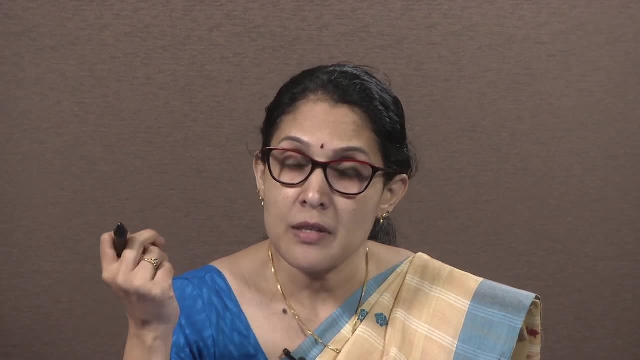 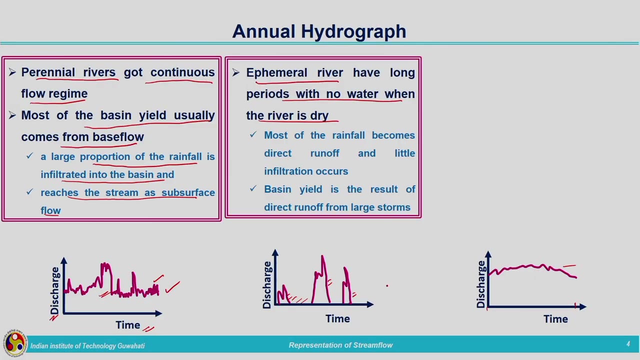 base flow component will not be there. even if it is present, it will be of small quantity. That is why certain period it is seen as dry. So because of this, the base flow component will not be there. So that is why certain periods it is super dry. 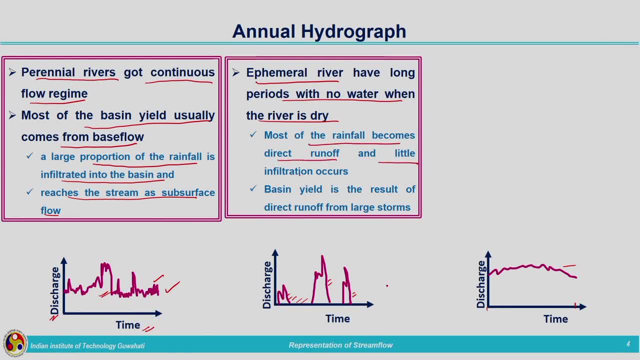 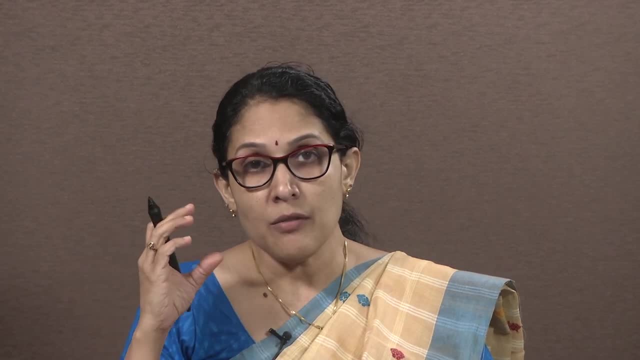 of the rainfall becomes direct runoff and little infiltration occurs, and basin yield is the result of direct runoff from large storms. In the first one we have seen, basin yield is from base flow, that is, the groundwater contribution. The second one from the curve itself, from the stream flow. 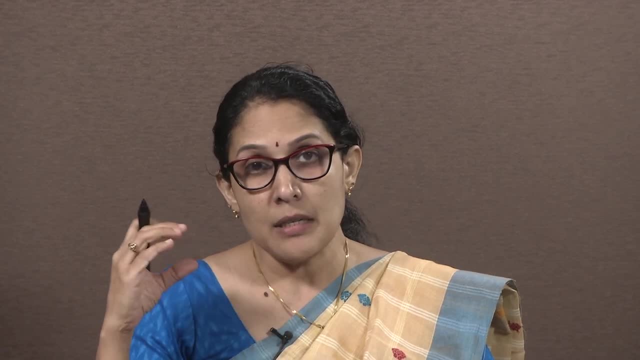 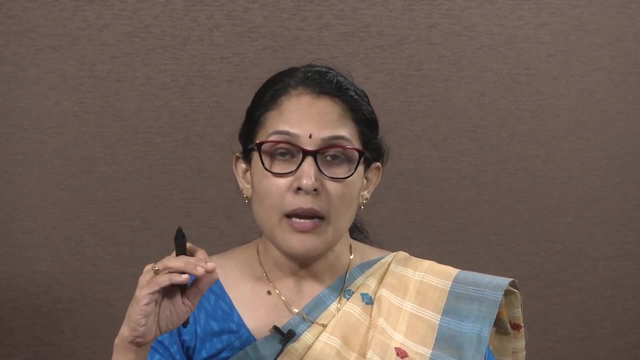 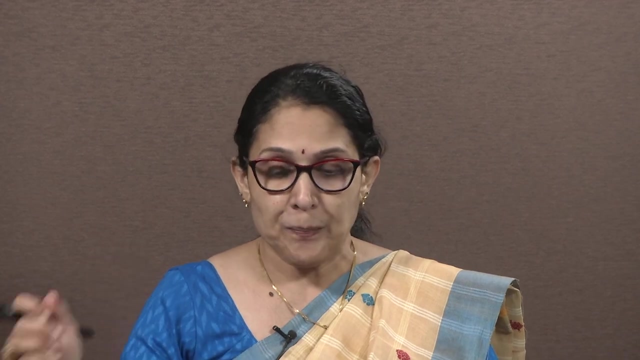 hydrograph itself. it is very clear that certain periods we do not have any water in the river. it is representing the dry season, in which the river is dry and the basin yield in such cases is coming from the surface runoff that is mainly from the storm. And in the case of third one, 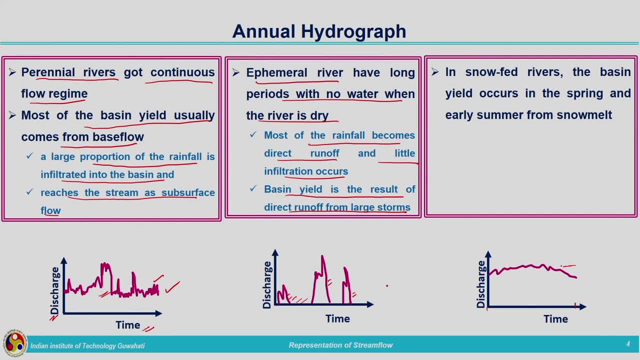 here you are observing almost there is not much variation in the flow value, So these are representing the case of snow fed rivers. The basin yield occurs in the spring and early summer From snow melt during summers and spring. because of snow melt, the stream flow will be observed. 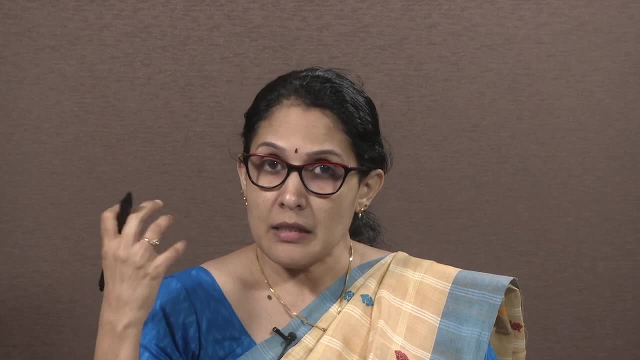 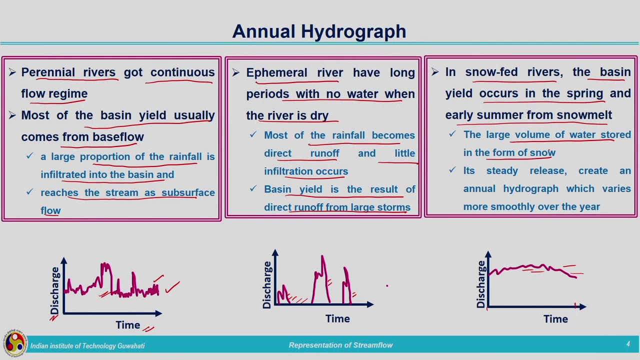 there at the gauging station, and this is mainly due to snow melt. The large volume of water stored in the form of snow, its steady release, creates an annual hydrograph which varies more smoothly over the year due to snow melt, and this is gradually released. 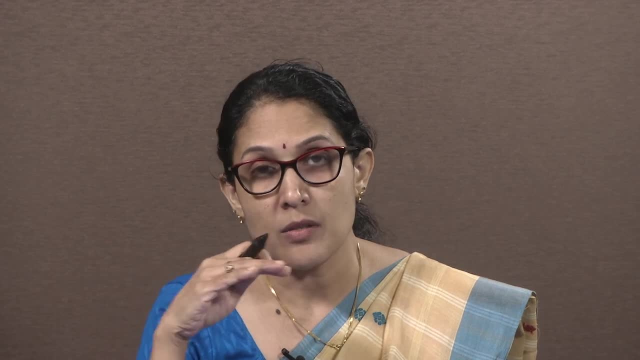 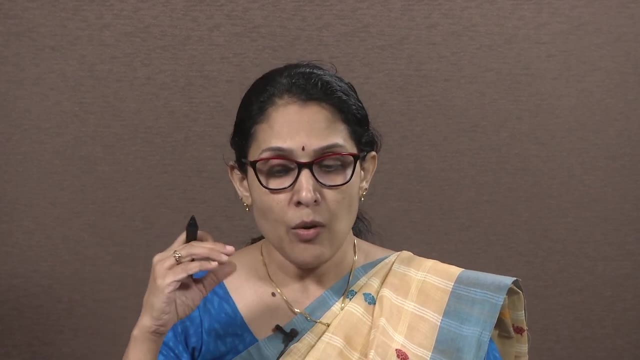 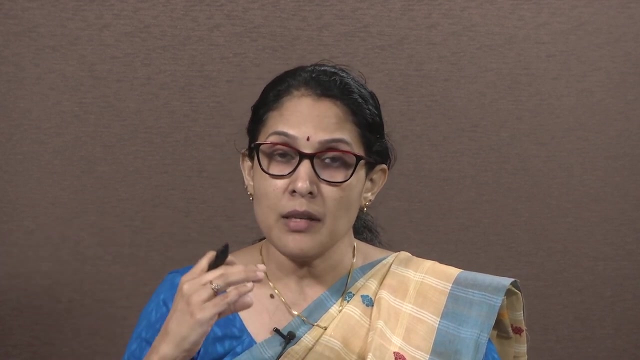 Because of the gradual release, the stream flow records are more or less uniform or smoothly varying over the entire period. I hope with these three representations it is clear to you what are the three types of annual hydrographs. In one, the basin yield is from the base flow. 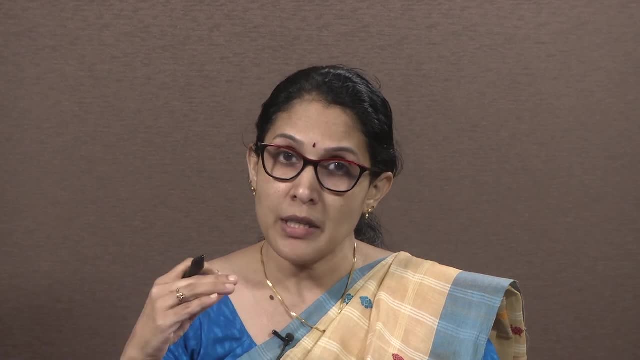 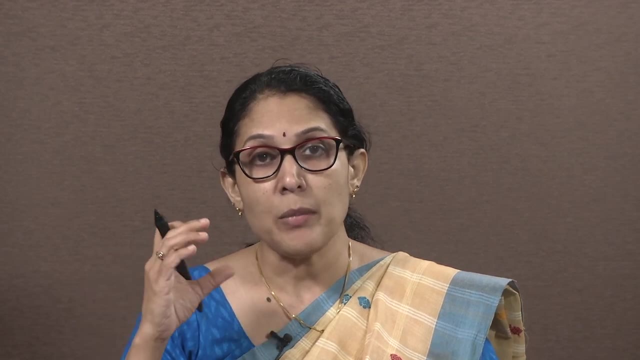 in such cases, we will be having flow throughout the year. that is the representation of perennial rivers. And in the second case, in the case of ephemeral rivers, we will be having flow throughout the year. In the third case, in the case of ephemeral rivers, we will be having the flow records. 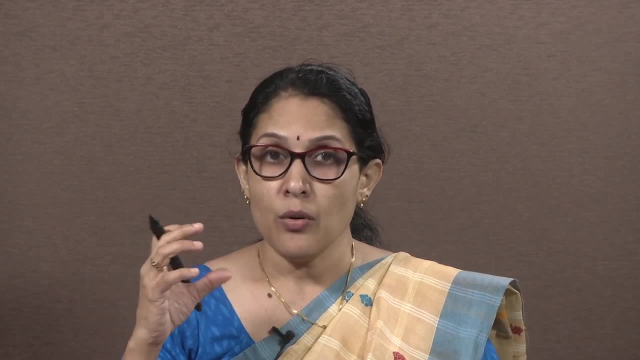 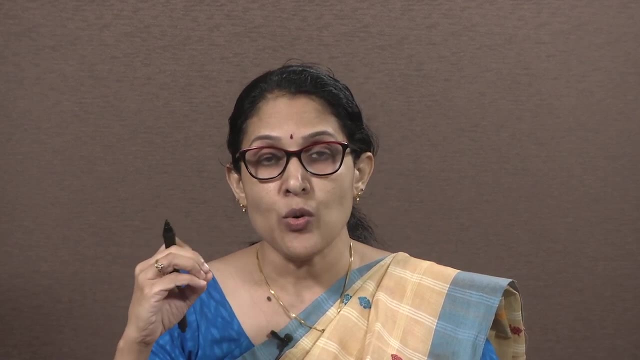 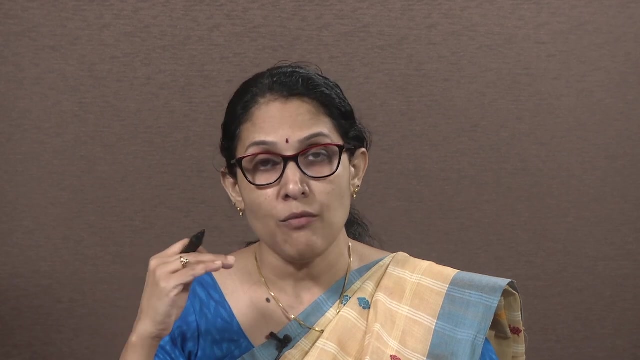 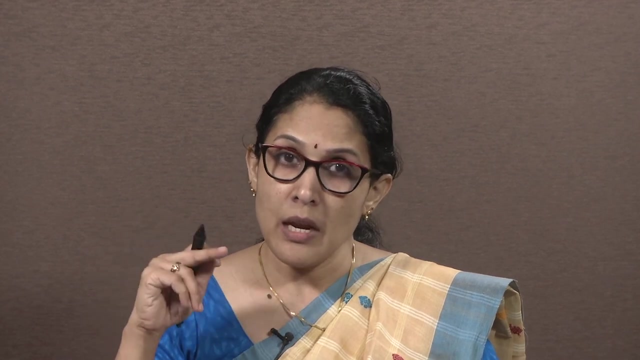 only during the monsoon season or whenever the precipitation is occurring- rainfall, especially rainfall is occurring- and other seasons. it will not be showing any stream flow data And in the case of snow fed rivers, there will be flow stream flow records, but it will be smoothly varying. there will not be any spikes due to rainfall present in those type of annual. 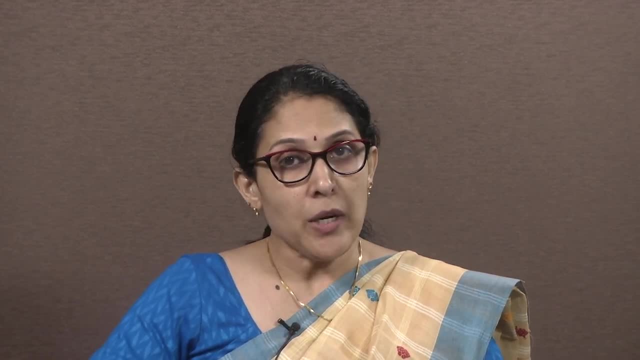 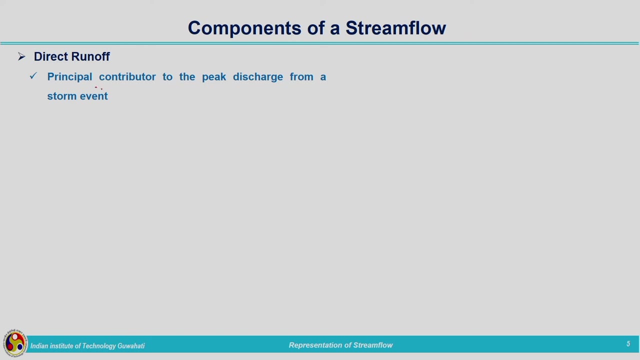 hydrographs. Now let us move on to the components of stream flow. First one is the direct runoff, and this is the principle contributed to the peak discharge from a storm event. During the storm event, you know what are the processes taking place. Initially, the catchment storage components. 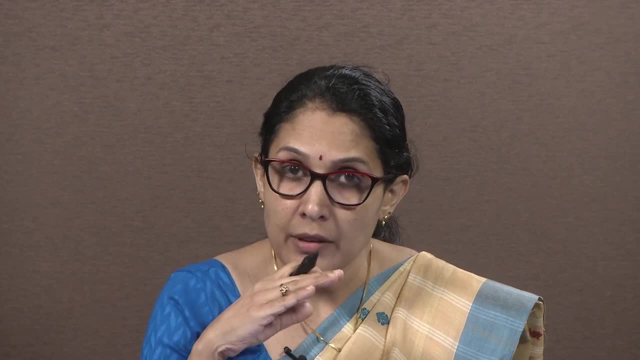 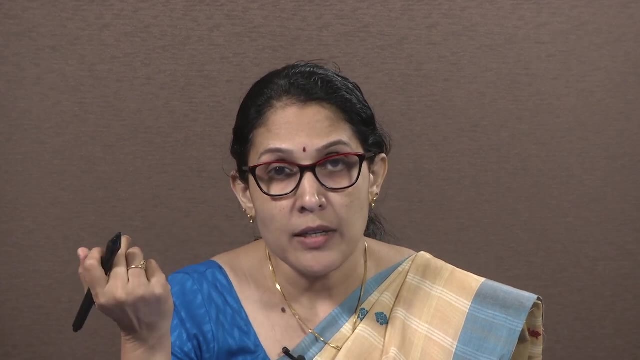 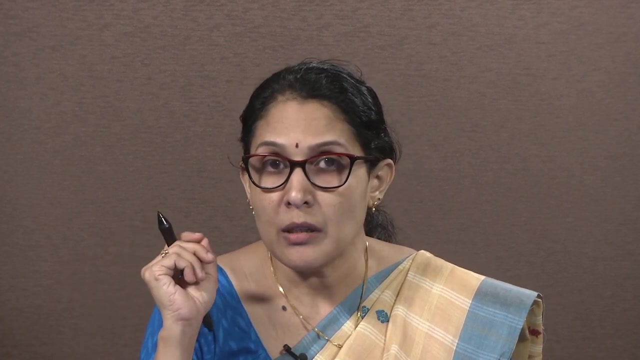 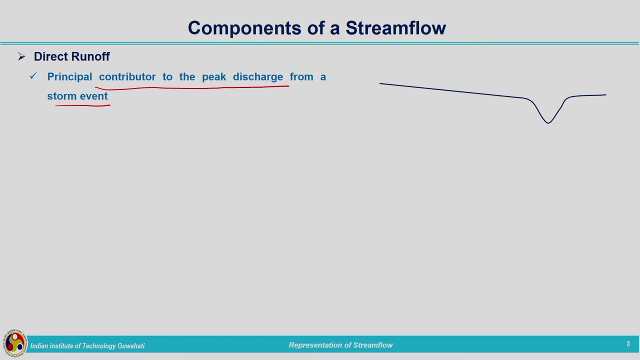 will be satisfied. after that we will be having the overland flow and it will be generated from altec and regurgistoire channel. Their flow will be starting out of a short skincare cycle of 24 hours andpopга flow results will be proper after. 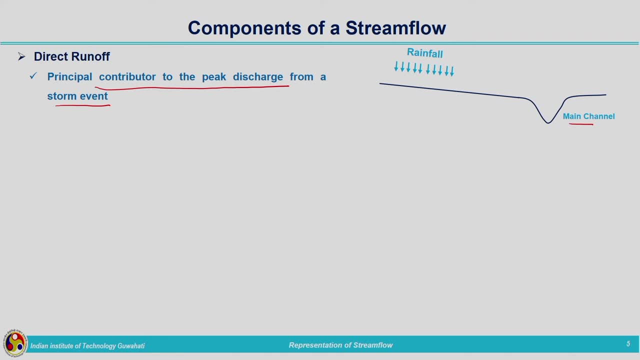 that we will have得到在the outlet ofthe basin joining channels and channel flow will be starting. finally, it will be contributions to the outlet ofthe basin. So the principal contributor to peak discharge is from a storm event, that is, from the direct runoff Skymetically. 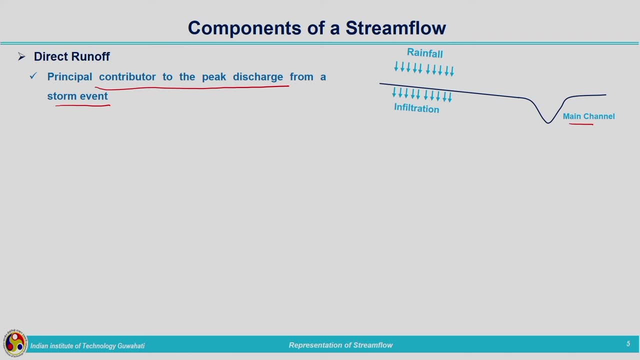 we can represent this. let this be the main channel And we are getting rainfall over the catchment And what will happen? infiltration will be taking place initially- And sir we will see- and other storage components also will be satisfied. After that we will be getting the 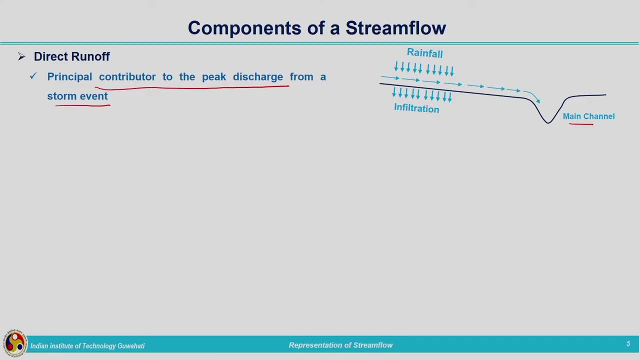 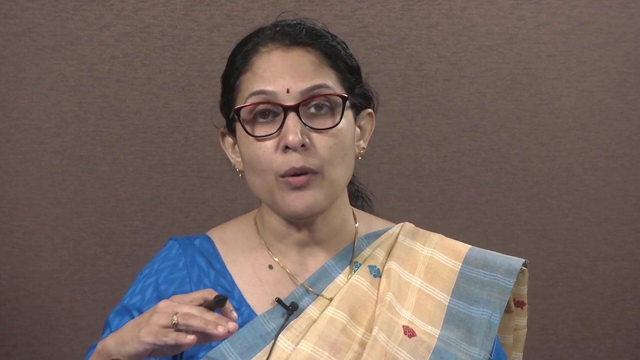 overland flow and channel flow. Finally, it will be meeting the main channel. in this way, It is the first to reach the channel, that is, rainfall is occurring, infiltration is taking place. Whatever remaining water, excess rainfall will be forming the overland flow and finally it 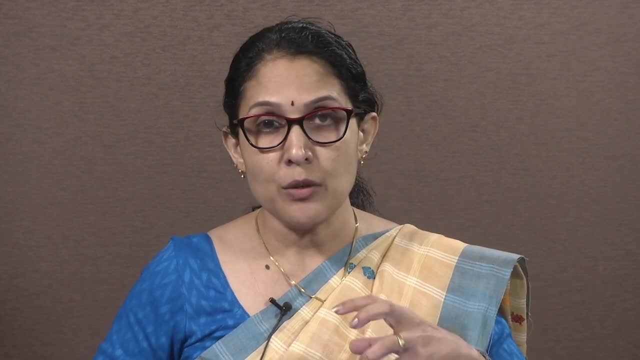 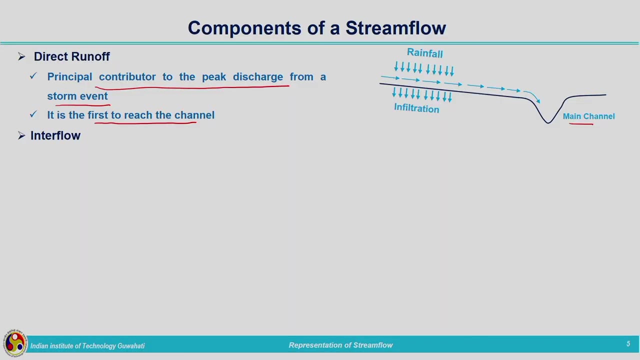 will be meeting the main channel. So this is the first one to reach the channel. and second one is interflow contribution from the subsurface. So movement of water is subject to more flow resistance. So when the flow is taking place beneath the ground surface, the resistance. 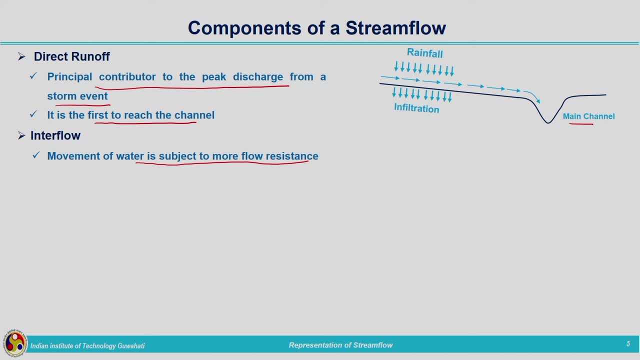 offered by the pores of the soil. pores will be more. It will not be as smooth as the overland flow. In this way, schematically, we can observe this: Precipitation is there and we are having the surface runoff and after the surface runoff started we will be having the interflow. 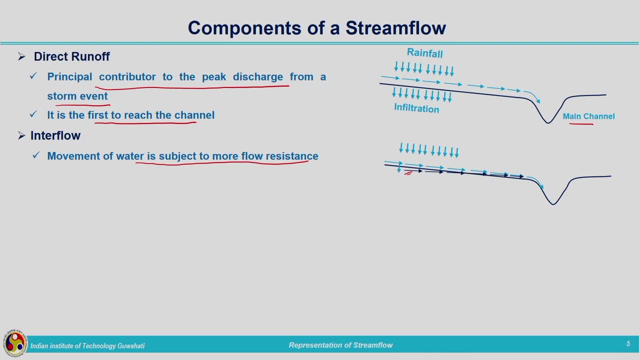 That is due to infiltration, water is moving into the ground surface and, because of the gradient, lateral flow of the subsurface water will be taking place and that also will be contributing to the overland flow. So this is the first one to reach the channel. 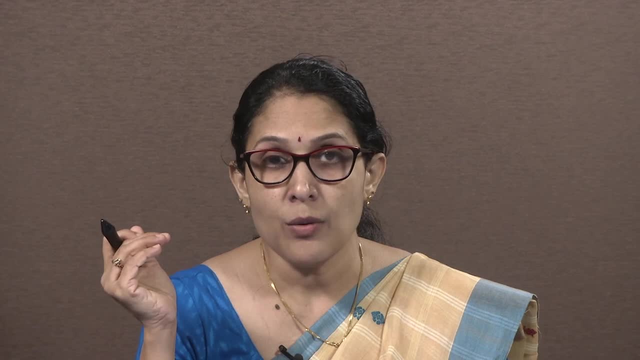 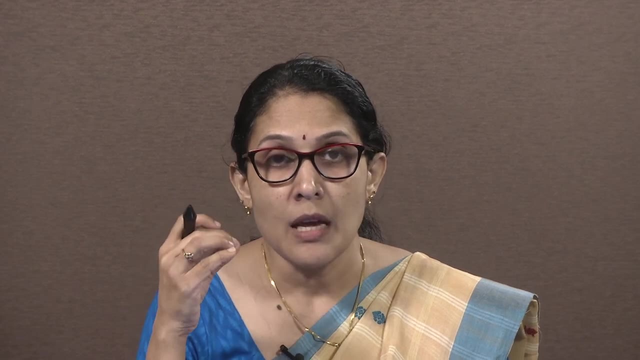 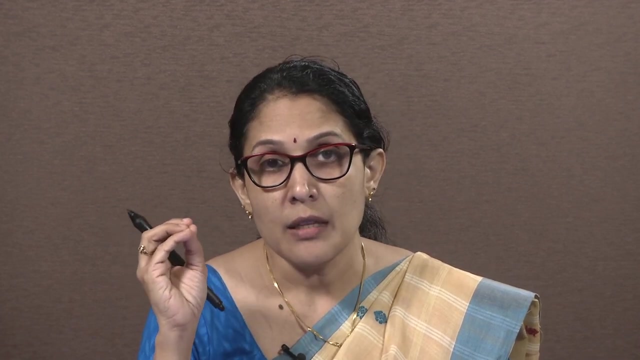 So the first one to reach the channel is contributing to the stream known as the interflow. So because of the resistance, more resistance for the flow beneath the ground surface, the rate with which it is flowing will be less compared to the surface runoff. That is why, at the beginning, we 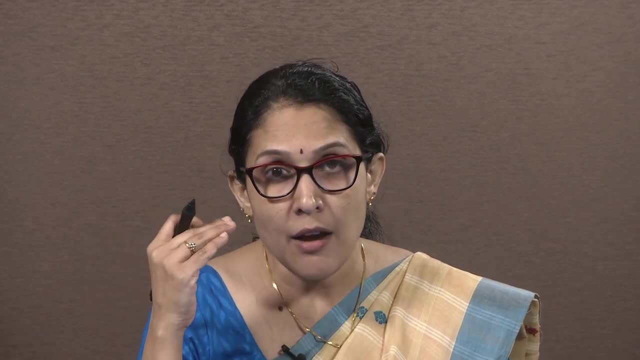 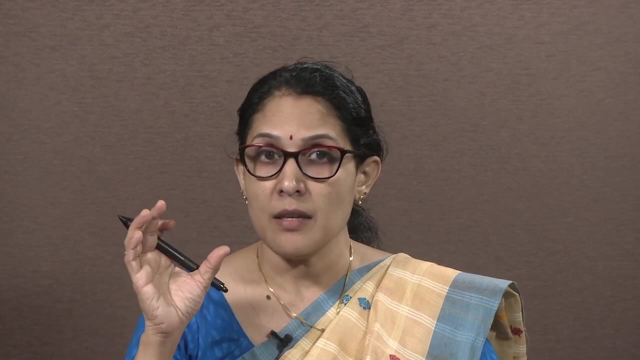 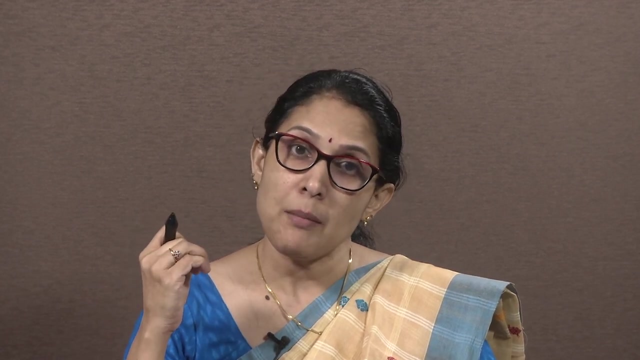 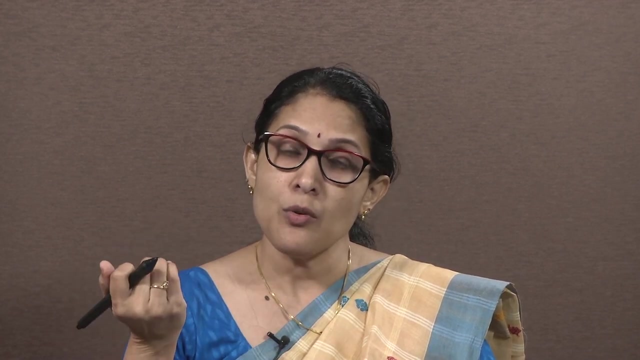 will be having the surface runoff and after certain time only the interflow will be starting. But there are certain cases We need to look into the catchment properties also Because if the interflow contribution is coming from nearby area of the stream, it can reach faster than the runoff contribution from the 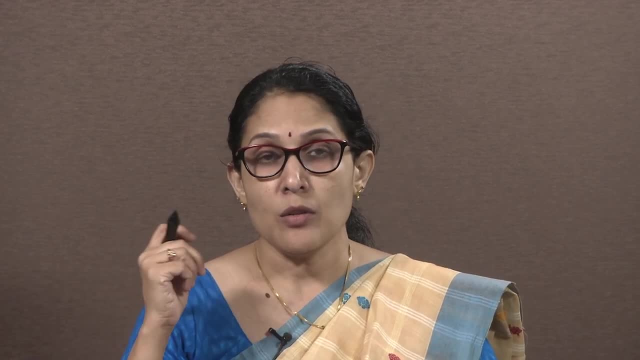 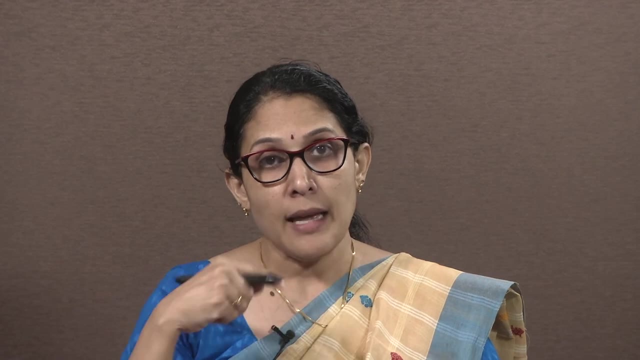 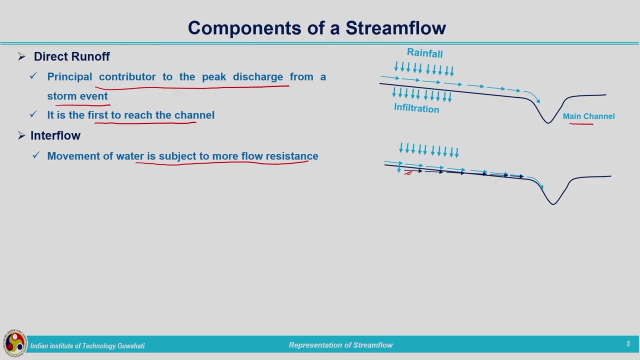 farther away point of the drainage basin. So the water which is coming as runoff from the farthest point will be taking more time than that of the interflow taking place from the nearby places To the channel. So in this case you can observe that we are having the surface runoff and at the 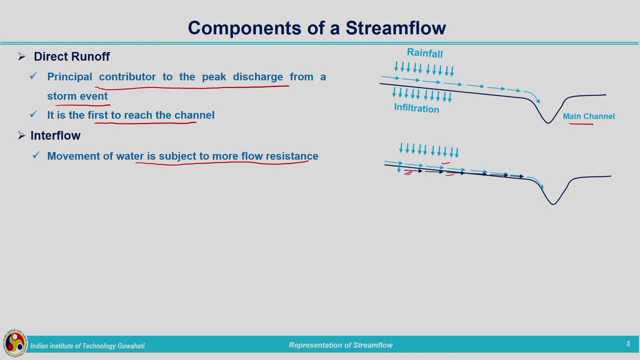 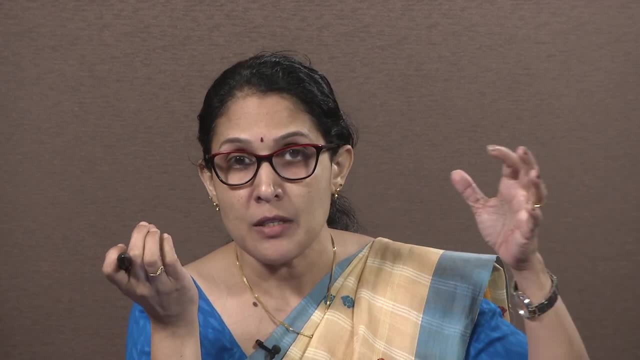 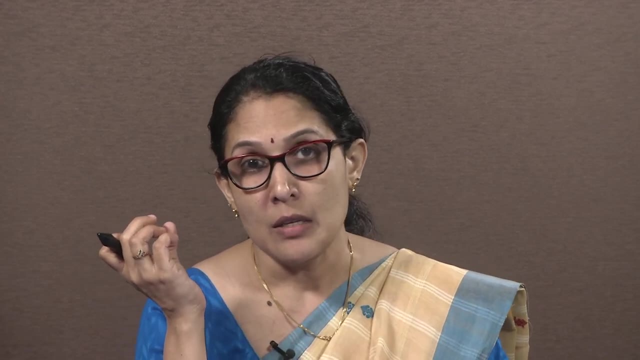 same time we are having interflow. Interflow is starting at a later time compared to surface runoff, But during the time when entire catchment is contributing runoff to the outlet point. By that time interflow also might have contributed to the stream flow. So these two together always. 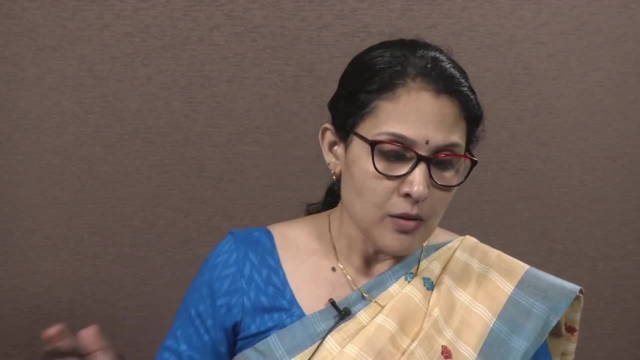 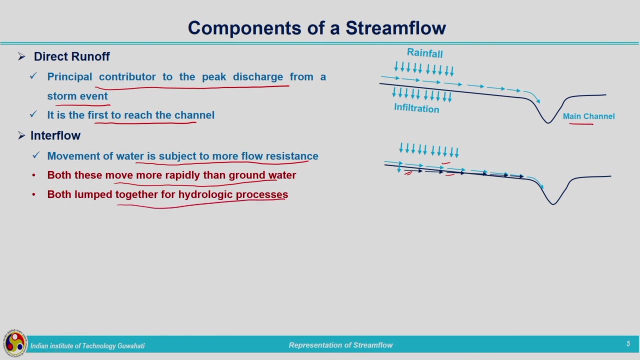 combined together When we discuss about Stream flow. stream flow, So both these move more rapidly than groundwater and both lump together for hydrologic processes. Even though three components are contributing towards stream flow, that is, the direct runoff, interflow and base flow, we will be combining direct runoff and interflow. 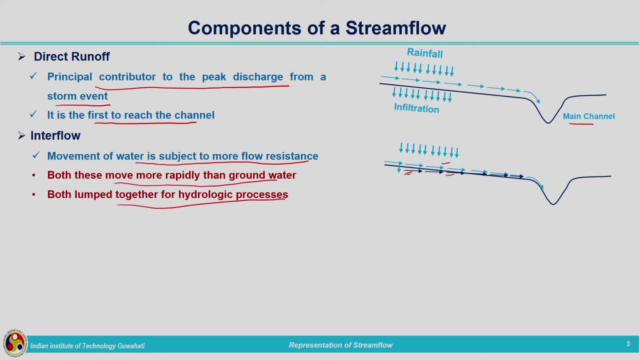 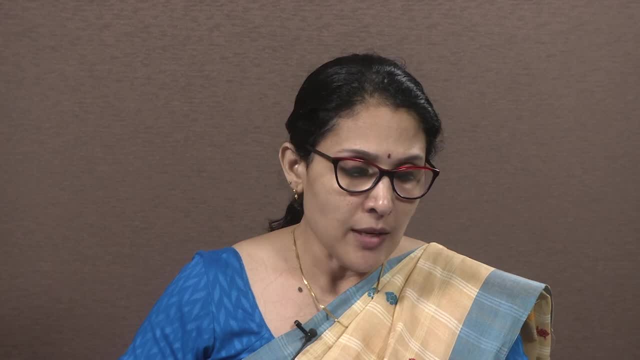 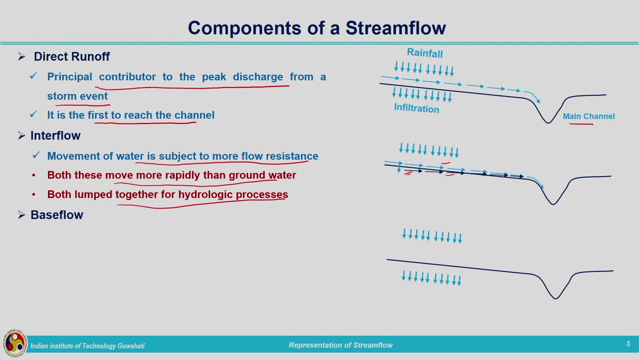 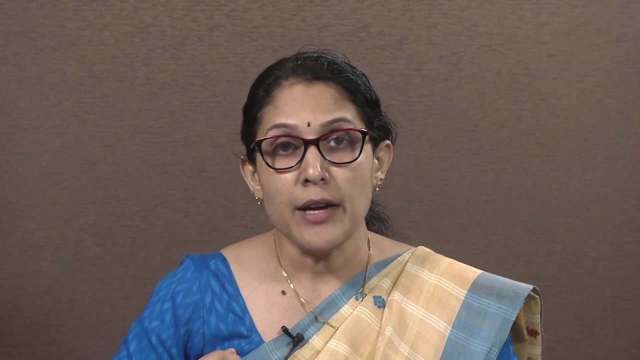 together because these two are moving faster, at a faster rate compared to base flow. that is the contribution from the groundwater. Now let us see the case with base flow. Again, the same schematic representation: rainfall is occurring, infiltration is taking place, This infiltrated water is percolating deeper into the soil and finally it will be meeting. 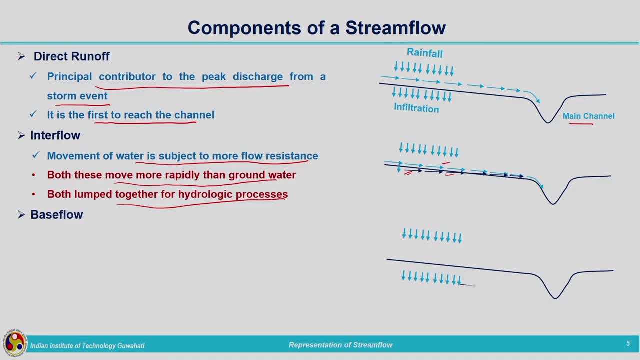 the groundwater table, Hence a contribution coming from the groundwater towards the stream. So the rate with which the base flow contribution is coming to the stream flow is at a slow rate and flow in a perennial stream prior to a storm is from base flow. We have seen the case with different annual 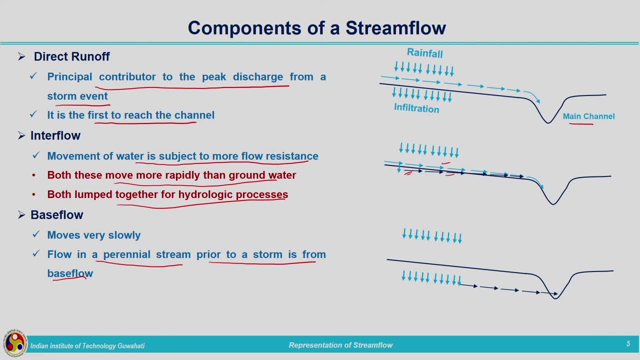 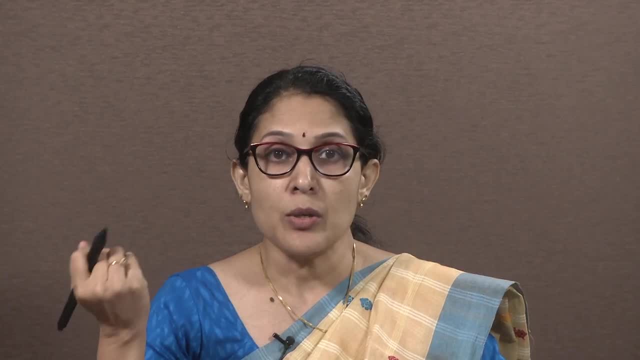 Hydrographs. in that case we have seen in the perennial rivers, all throughout the year there will be stream flow or water present in the river. So that is mainly due to the contribution from base flow. But this base flow is not contributing to peak discharge for a given. 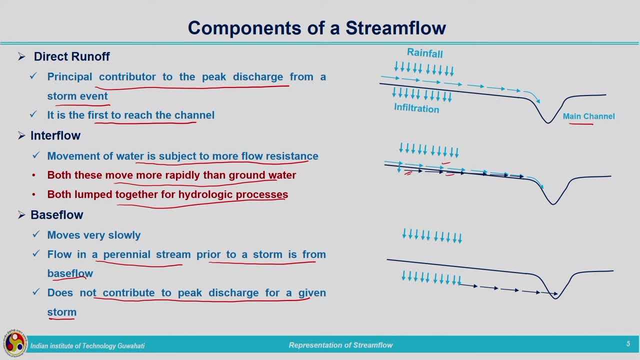 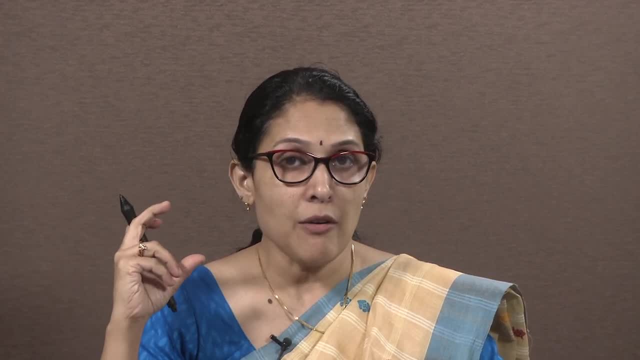 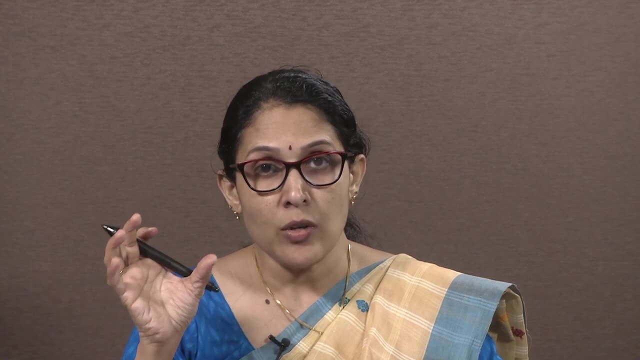 storm. given storm, the peak discharges mainly from the surface runoff. Now let us see different components of storm hydrograph. Different hydrographs which we have observed are annual hydrograph and also storm hydrograph. So for a particular period, shorter period during the time of storm, and just 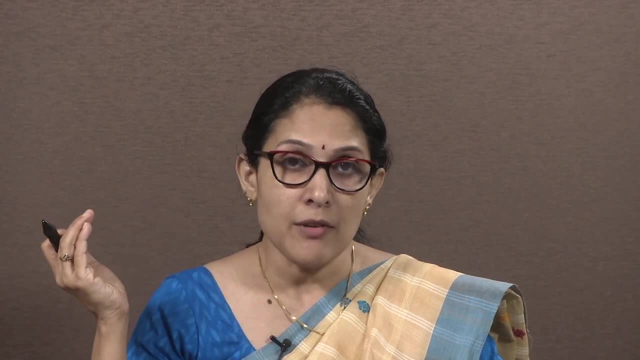 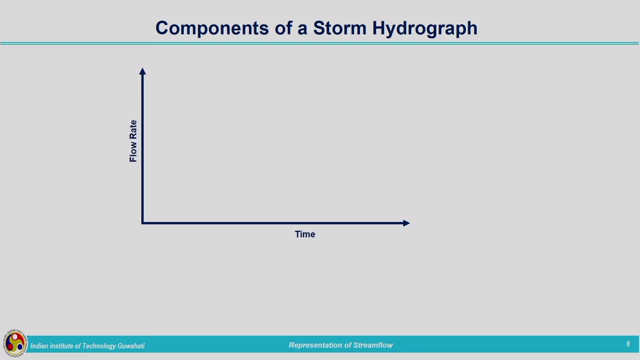 after the storm, the flow records are plotted. that is our storm hydrograph. So now let us look into the components of storm hydrograph. So this is a storm hydrograph. We are plotting flow rate along the y axis or the discharge along the y axis. Different names are the flow rate, discharge. 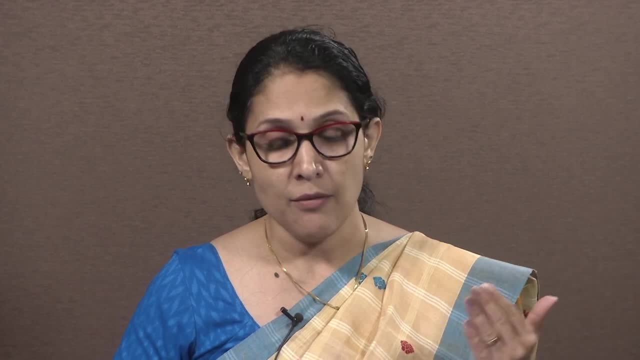 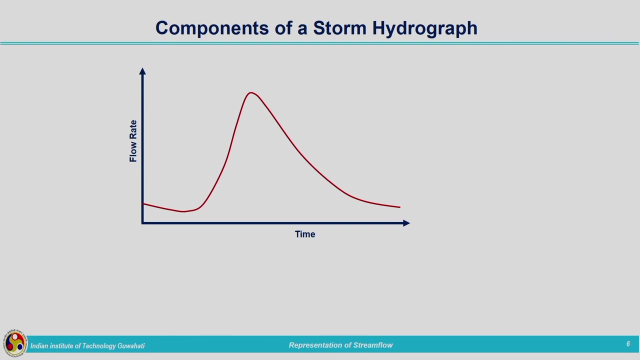 stream flow. whatever way you are calling it, is plotting along the y axis and time along the x axis. This is a schematic representation of hydrograph. You always the hydrograph will not be looking like this. It will not be a smooth curve, because you imagine. 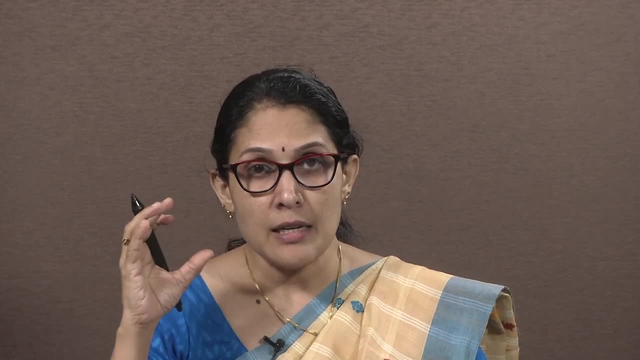 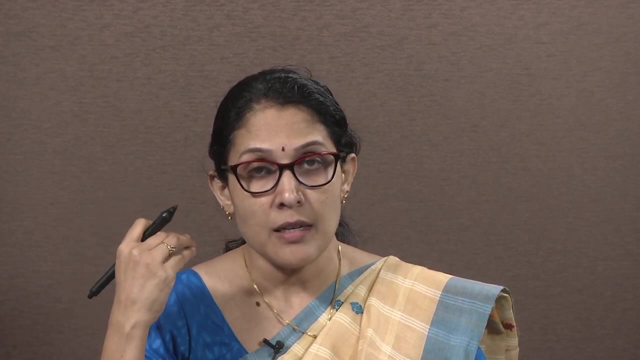 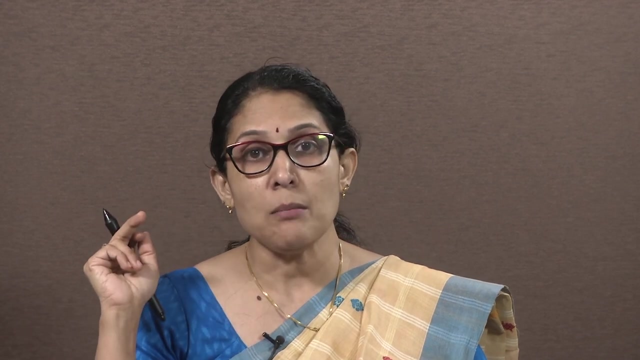 the case of a stream where the water from different channels are meeting. In such cases, one channel will be contributing first, other one will be coming at a later stage, So that there will be spikes when we observe the stream flow data. It can be smoothened by. 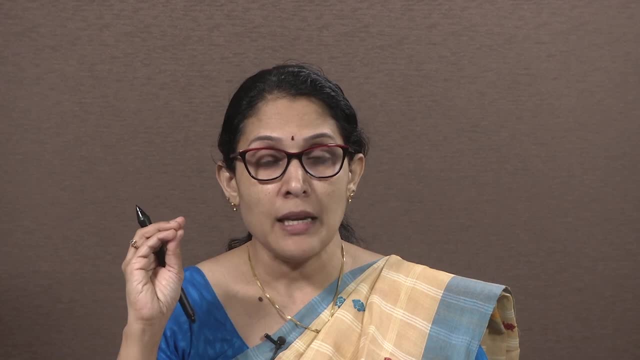 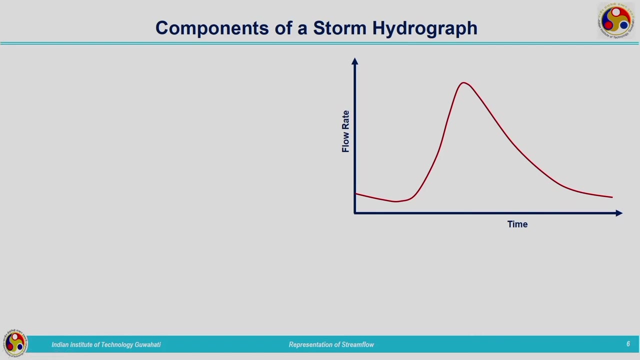 means of different techniques, but usually we will not be getting a very smooth curve like this. So we can see different components of the storm hydrograph with the help of this figure. So it is starting from the point A and up to B. You can see there is a recession taking place. 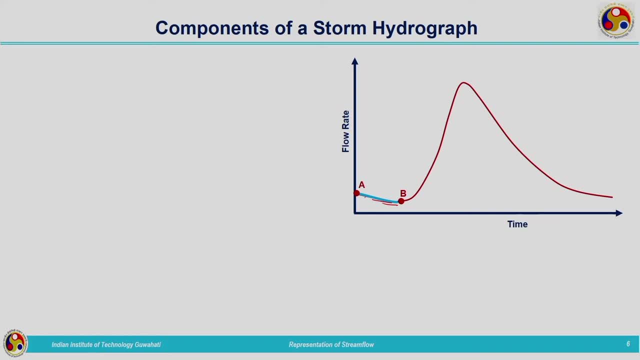 and from this point B onwards it is increasing. So prior to the time of intense rainfall, contribution is from base flow. That is represented by this segment AB. Even though there is no rainfall, we will be observing flow, So that is from the base flow contribution. That is the. 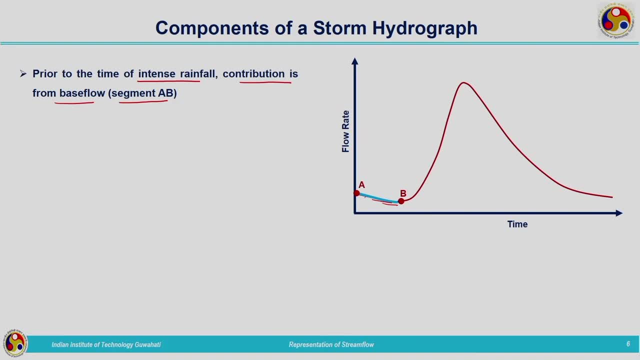 flow contribution. So that is represented by this segment, AB. AB is termed as the base flow recession. Now, from B to C you can see it is rising. From B onwards the runoff is started and it is rising and BC is called rising limb of the hydrograph And BC is representing when. 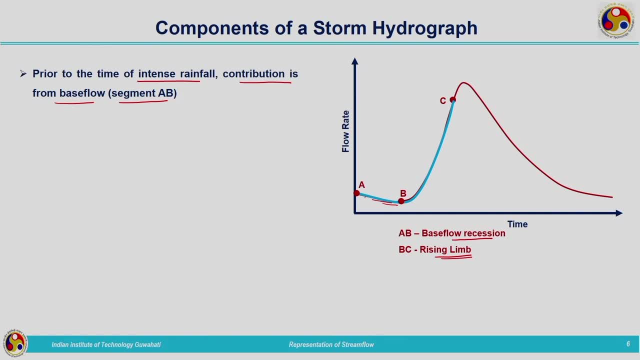 the increase in flow rate is taking place. Increase in flow rate means there is contribution coming from runoff. That is, after satisfying the storage components, overland flow started and contribution of runoff has reached the outlet point. So this BC is the representation of the storm characteristics and also catchment characteristics, And then from that it is. 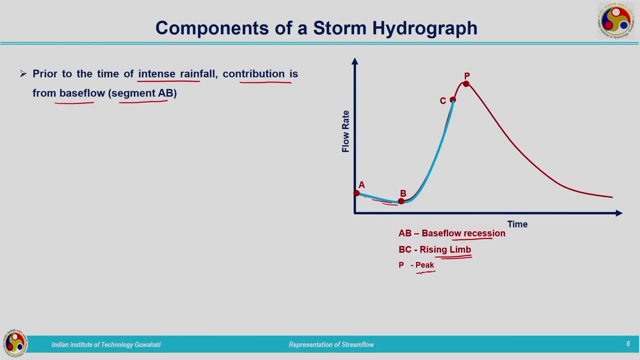 peaked up to point P. P is representing the peak of the hydrograph. Then you can see, it is dropped down to point D. So CPD is representing the crest. Actually, we cannot expect a sharp peak. That is expected only in certain watersheds, Since the peak value is consisting of the 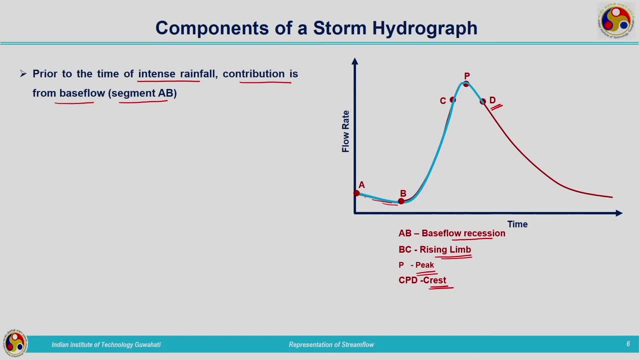 contribution from different areas of the watershed. it may be having certain spikes present or fluctuations present, So that part is represented by the crest and the peak point from that is the hydrograph peak. So CPD is representing the crest And from D the recession in the flow is. 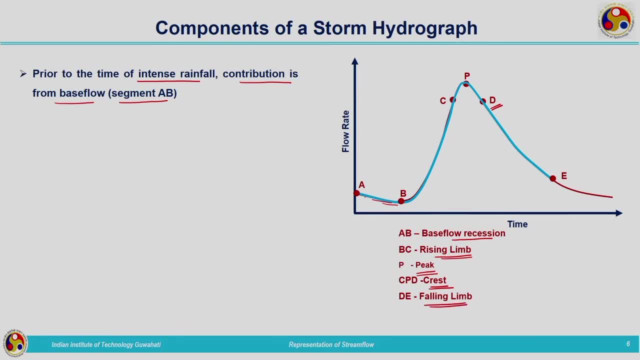 taking place. That is representing the falling limb. DE is representing falling limb, That is, there is a recession in the flow is taking place. Then from E to F, again it is representing base flow recession. When it reaches the point D, all the contribution from runoff is stopped. 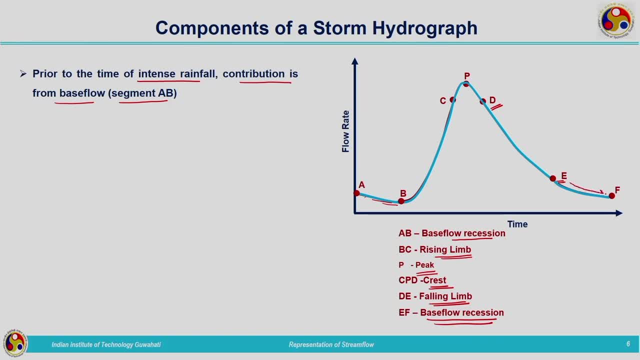 Only the contribution related to this part is from base flow. That is termed as the base flow recession, And D is a point of inflection. So here I have told you. the crest is represented by CPD. So what is meant by this point D? D is the point termed as point of inflection. That point is very. 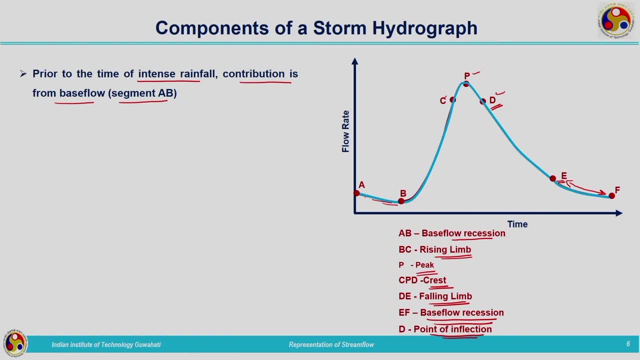 important because this point is considered as the time at which all the flow of the water is being done and all the storage components are completely satisfied. Once it reaches this point, by this time already the storm has stopped and the entire cachemun is started to contribute. 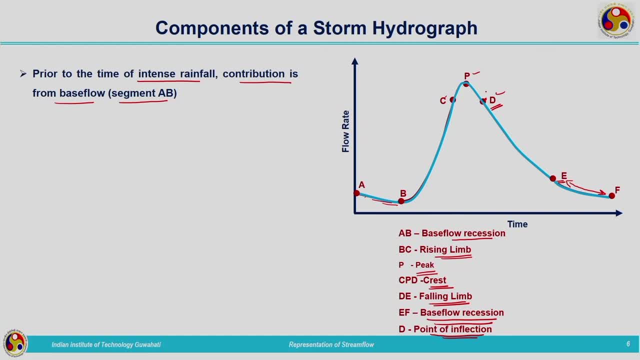 flow towards the outlet point. After that, what will happen? recession in the flow takes place, that is, the withdrawal from the storage will be starting beyond this point D. Direct runoff begins at B, peaks at P and ends at CPD. So you can see BPE. the direct runoff is from B to E. The peak is occurring at the point P. 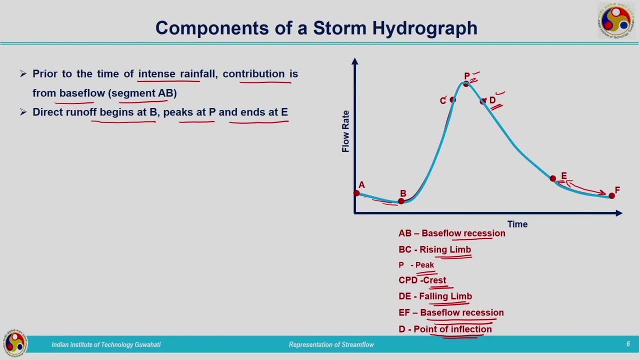 So, depending on the characteristics of the catchment, we may have the sharp peak or flat peak. Then basin and storm characteristics control the shape of the rising limb. because I have already told you, B is the point where the runoff starts. So the shape of the rising limb is 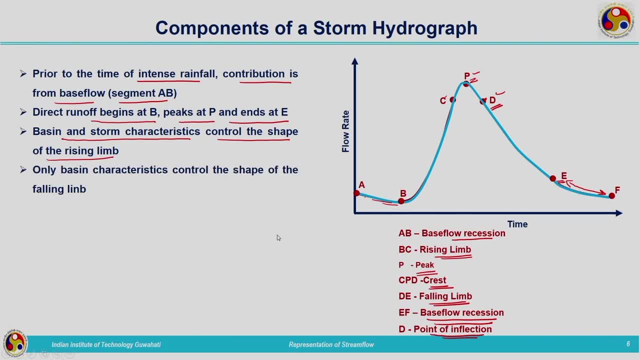 characterized by the basin and storm characteristics. Then, coming to the falling limb, the shape of the falling limb depends only on the basin characteristics because by the time the peak has attained, the storm has already stopped. So when we discuss about the shape of the falling limb, there is no contribution coming from storm characteristics. It is purely based on. 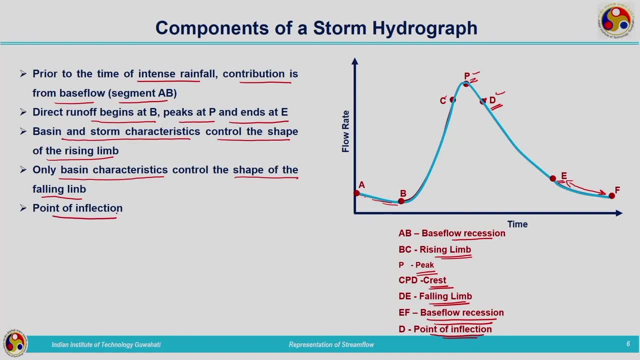 the basin characteristics. Now coming to the point of inflection. Point of inflection is the starting point of the recession limb. Recession limb is also termed as falling limb. So the point of inflection is nothing but the starting point of the recession. 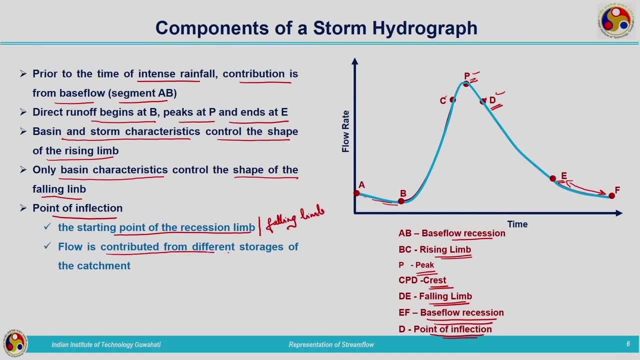 limb. So at this point the flow is contributed from different storages of catchment and after this the withdrawal of the flow from the storages will be taking place and this point of inflection is representing the point of maximum Storage. I hope different components of storm hydrograph is clear to you. This thing should be. 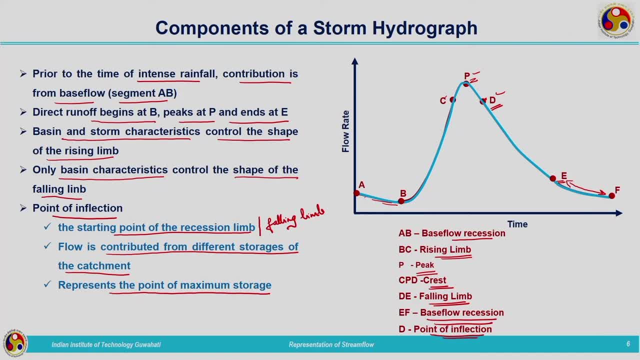 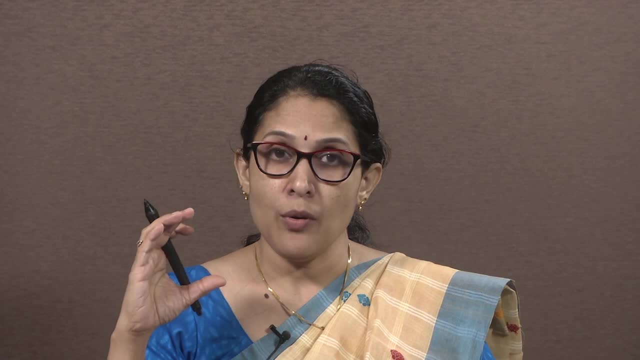 very clear when we move on to the hydrograph analysis. That is the next module. So the components of hydrograph is important and regarding the time related components, we will discuss at the time of hydrograph analysis. When we talk about the stream flow, it is the 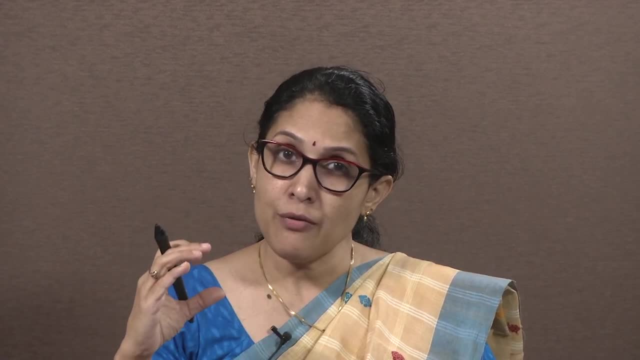 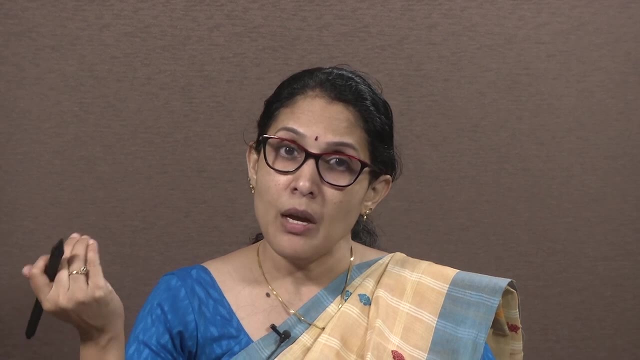 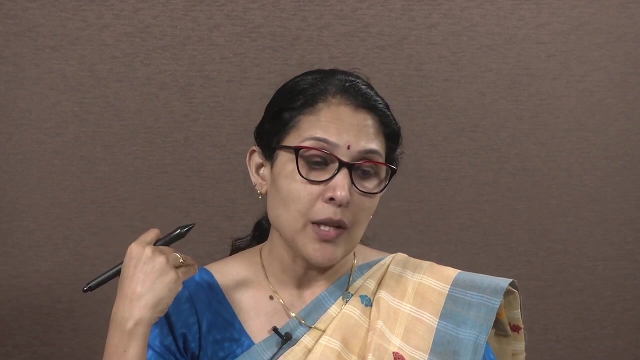 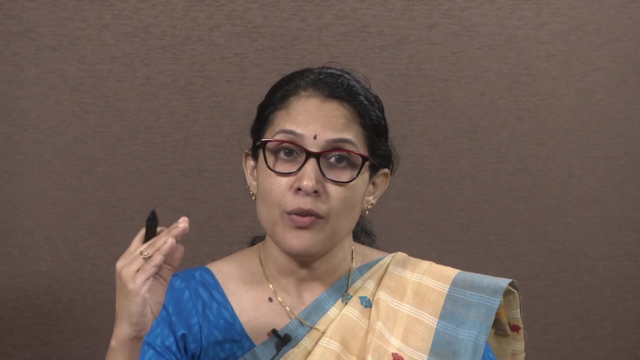 contribution from surface runoff, interflow and base flow. Since base flow is taking too much of time to contribute towards stream flow, we have combined surface runoff and interflow together and base flow separately. So whenever we are doing the study related to surface runoff or excess runoff, we need to separate the base. 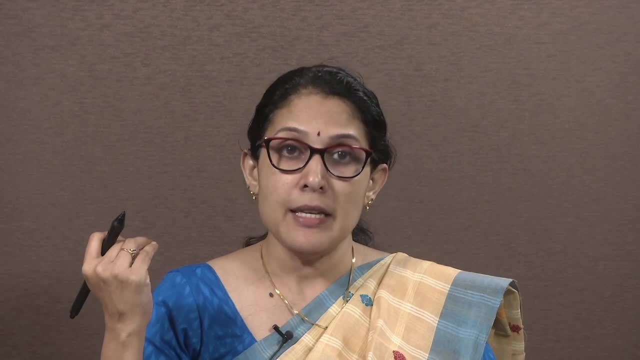 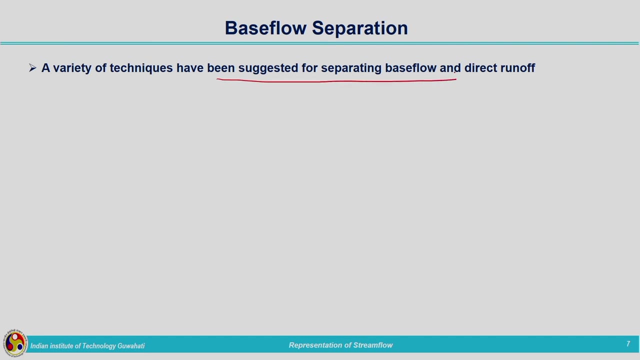 flow contribution. So for that different techniques are available. Let us see one by one. Variety of techniques have been suggested in this research for the external flow. So for the suggested for separating base flow and direct runoff, that is, what is the contribution coming from groundwater and also from the surface flow and interflow that we need to separate. 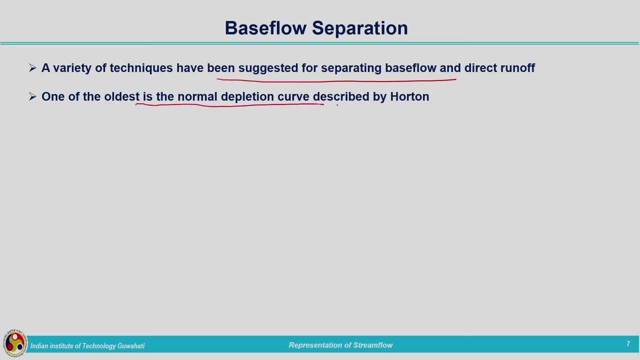 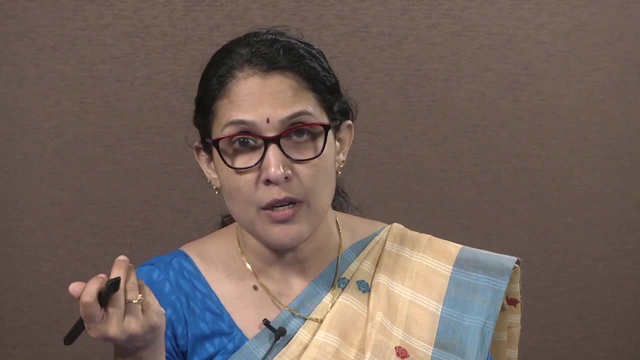 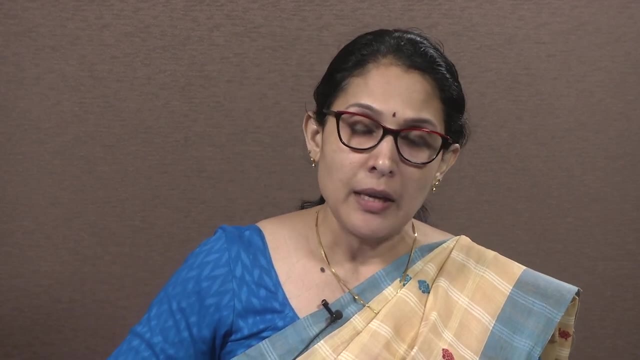 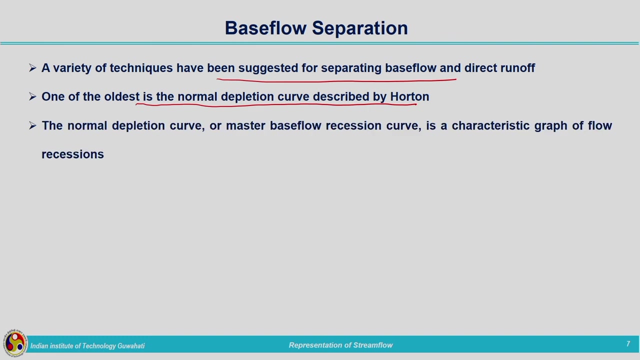 So one of the oldest method is the normal depletion curve described by Horton. Horton has carried out studies related to stream flow, surface runoff, interflow and all, and he has proposed the normal depletion curve. That normal depletion curve method can be utilized for base flow separation. So what is this normal depletion curve? Normal depletion. 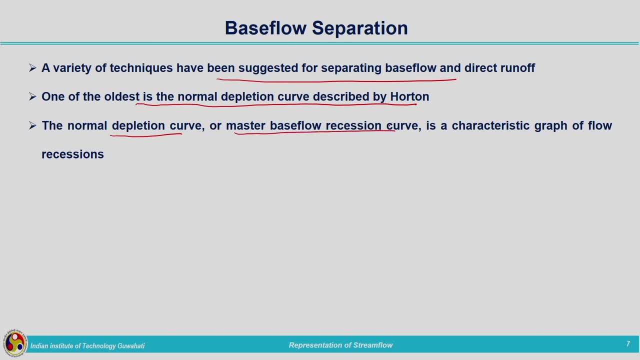 curve or the master base flow recession curve. it is a characteristic graph of flow recessions. It is representing the flow recessions. So recessions curve have been represented by means of an exponential curve. So the recessions curve is represented by an exponential decay, which is given by the 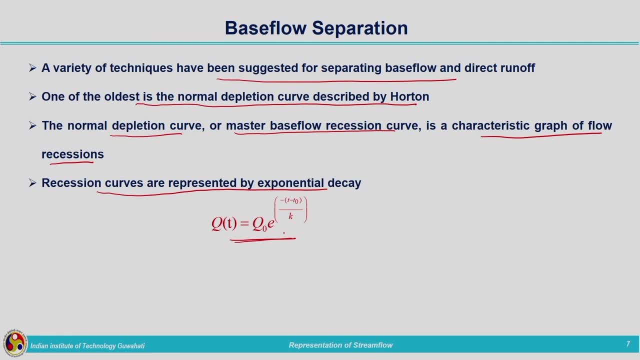 formula Qt is equal to Q0, e to the power of minus T, minus T0 divided by k. So the recessions curves have been represented by an exponential relationship that is given by this. It is proposed by Horton and in this Q0 is the flow at time, T0 and k is the exponential decay. 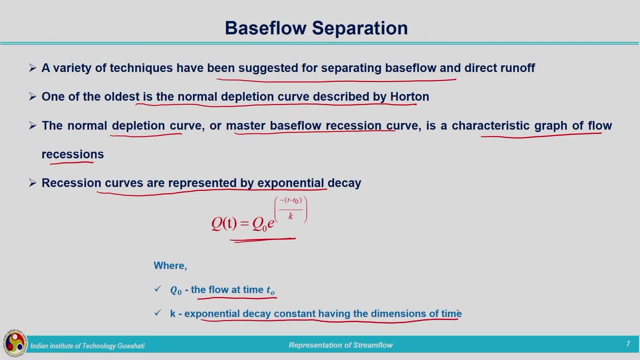 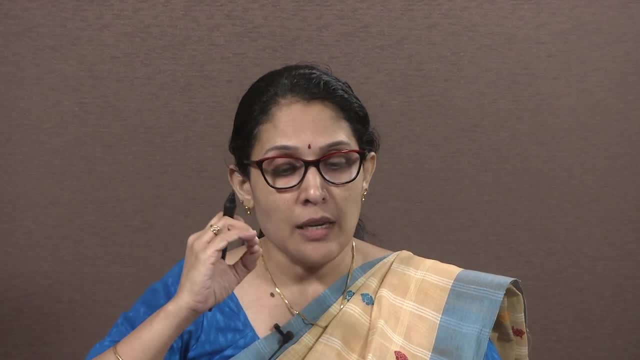 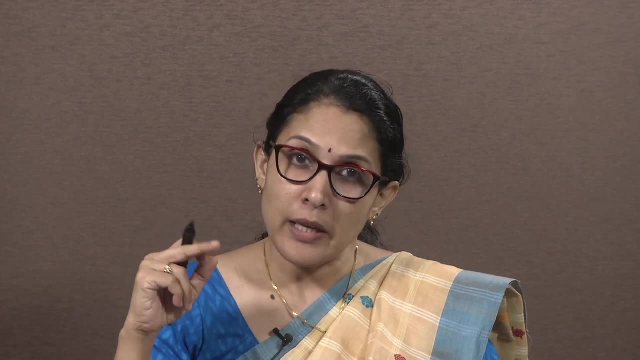 constant, having the dimensions of time. So for different times, T minus T0, T0 is the beginning of the storm and T for different time- we can get the ordinance related to this recession curves. So this equation can be utilized for plotting the recession curve. 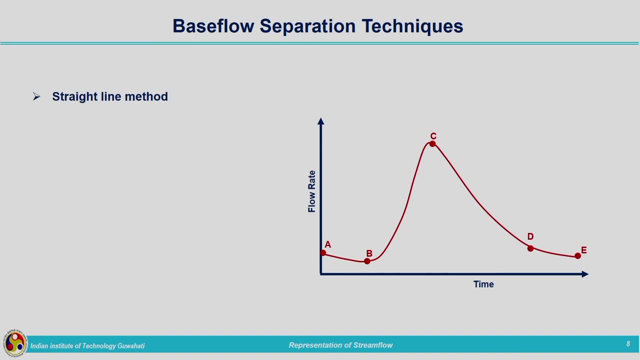 Now let us move on to base flow separation techniques. Different techniques are the straight line method, fixed base length method, variable slope method. So we are having the storm hydrograph over here And let us see different methods for separating the base flow from direct runoff. 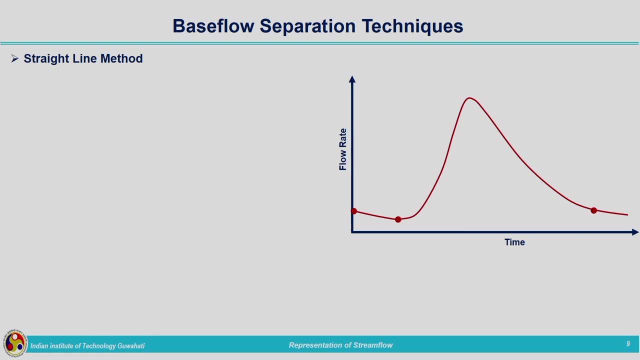 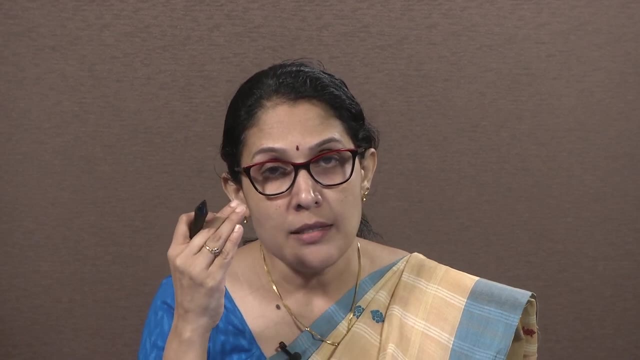 First one is the straight line method. In this, what we are doing, a horizontal line is drawn from the point at which surface runoff begins to the intersection with the recession limb. Initially, we will be having base flow contribution only and base flow recession will be starting. 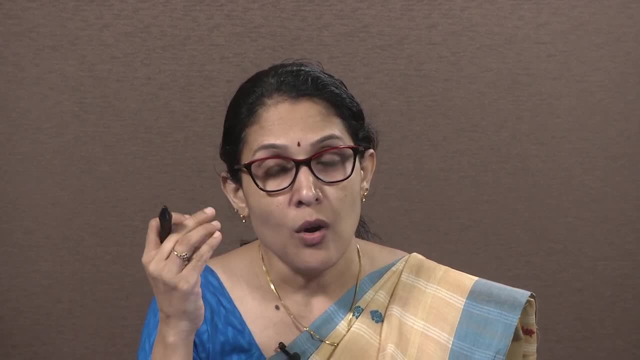 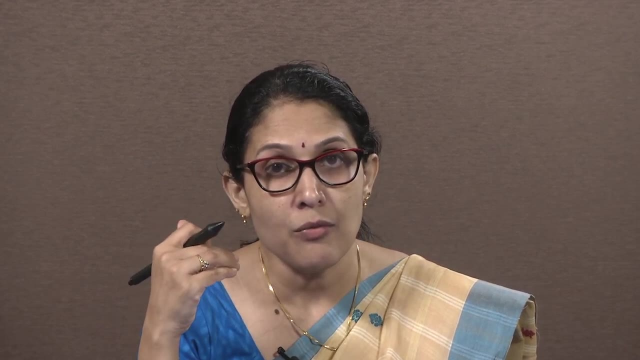 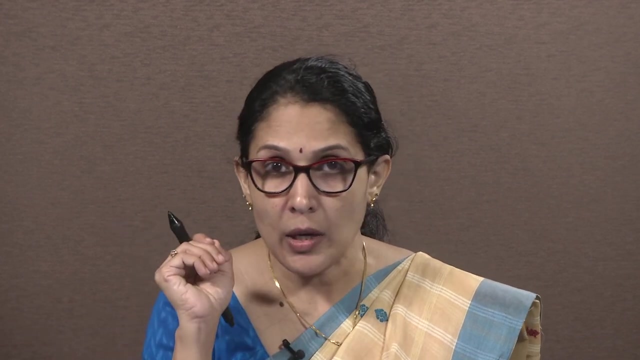 and at the time of storm or at the beginning of storm Also, there will not be any contribution from rainfall. As all the storages get satisfied, the contribution from rainfall towards the stream flow starts and the rising limb starts. So that particular point is the- represented over here- beginning of the rising limb. 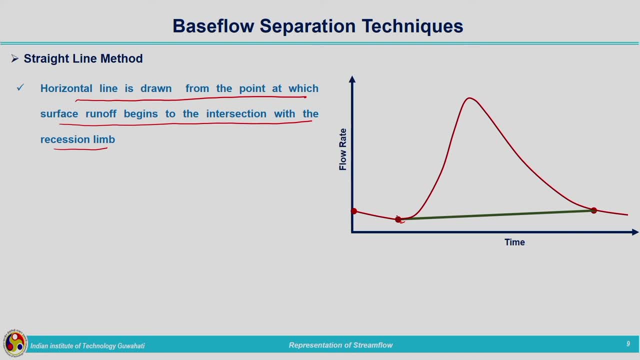 So what we will be doing, We will be joining the beginning point and the end point where the recession occurs. So we will be joining the beginning point and the end point where the recession occurs. And we will be joining the beginning point and the end point where the recession occurs. 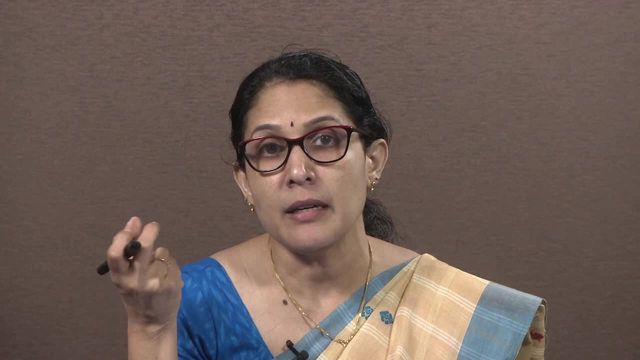 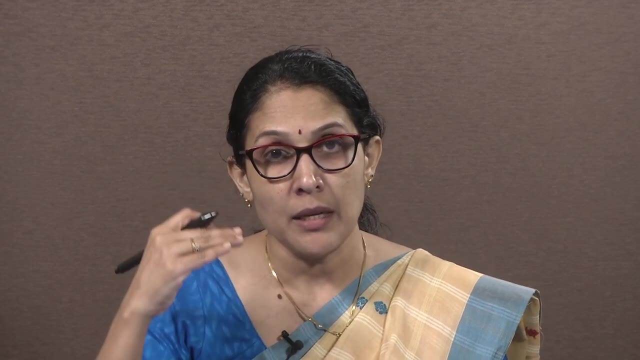 So all these points will be connected by the straight line method, making sure that at the beginning point the curve is ending and only the base flow contribution will be there. after that, Those two points will be connected by means of a straight line and beneath whatever coming beneath that straight line, whatever is present, that will be deducted from the 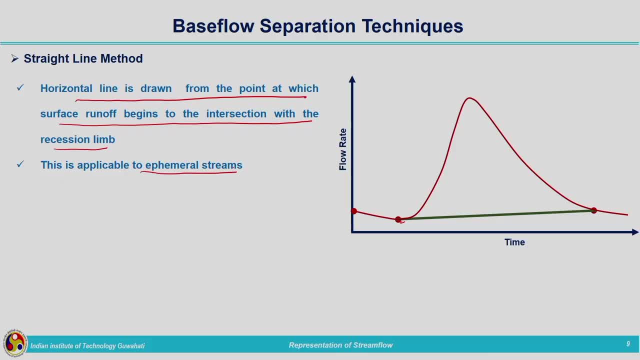 total flow. So this is applicable to ephemeral streams. And an improvement over this method is to use an inclined line to connect the beginning point of the surface run off with a point on the recession limb. So the green line will on the recession limb of hydrograph, where normal base flow resumes back. 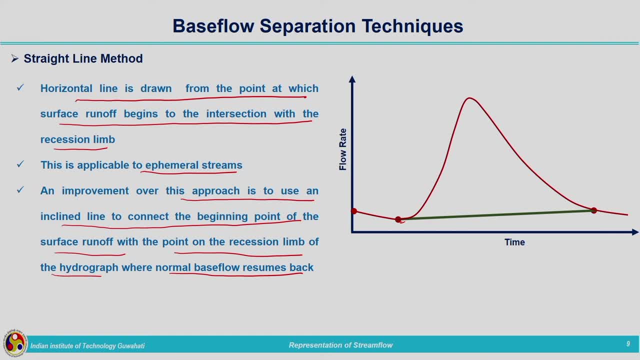 Instead of joining by means of a straight line, we can have an inclined line. also For small forested watersheds in humid regions this method can be applied, But always this is an approximate method. always it will not be giving you the accurate value. 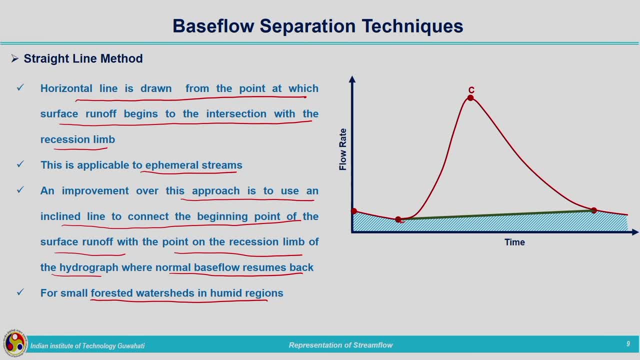 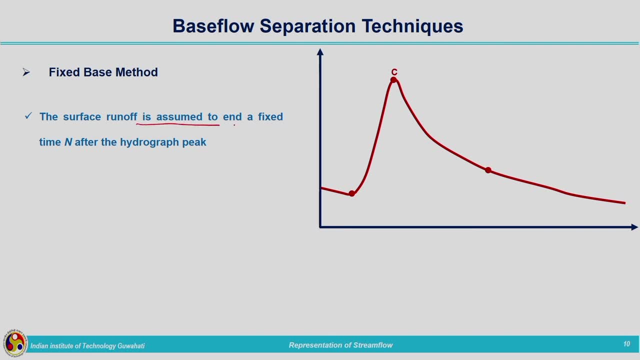 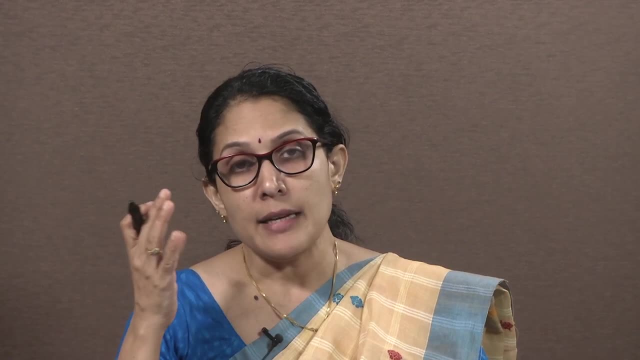 So these hatched portion is representing the base flow. So now, in the case of fixed base method, what we are doing? the surface runoff is assumed to end at a fixed time end after the hydrograph peak. Hydrograph peak when it is occurring, entire catchment is contributing water towards the 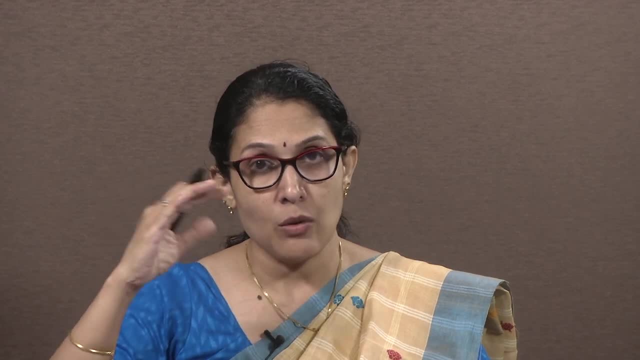 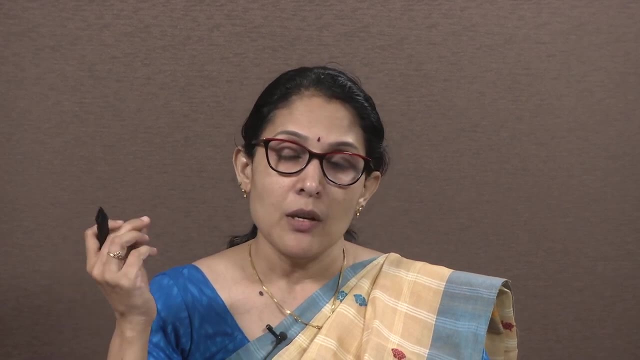 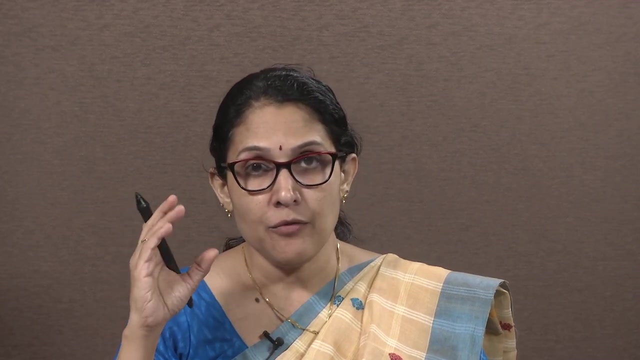 outlet point. So then we may be getting a flat peak or sharp peak, depending on the storm characteristic and also the basin characteristics. So what we are telling? The storm runoff will be stopped after a fixed time from the peak. That let us see schematically. 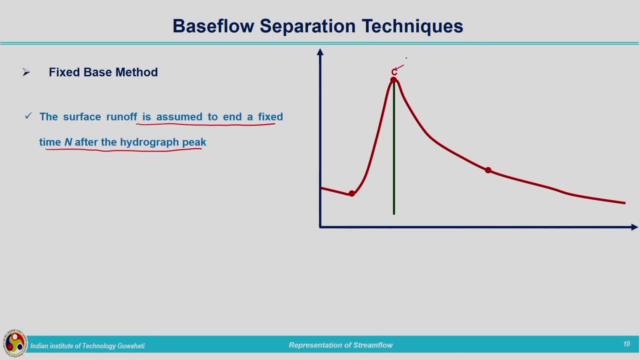 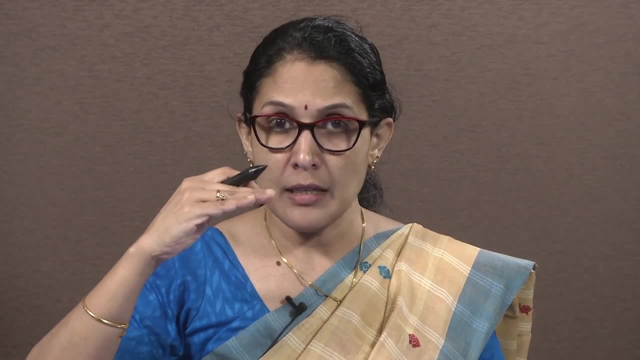 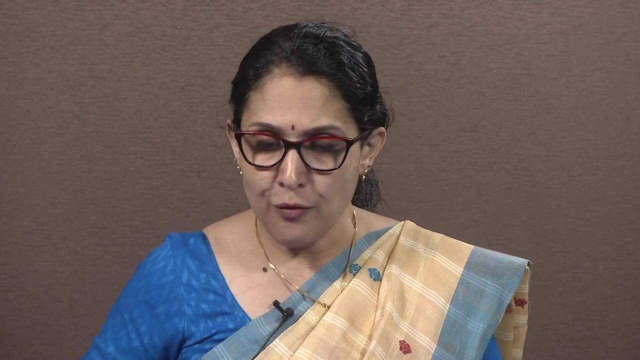 So C is representing our peak. It is approximated by means of a single peak point. It may be a flat peak also, So in that case you can consider the ending of the flat or the central point of the flat region. So from there we are considering certain conditions. 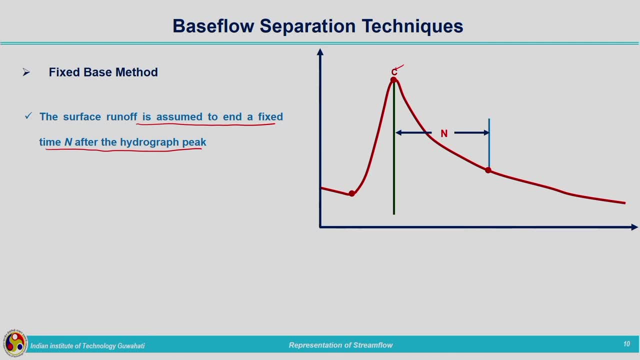 Let us see. So what we are saying is we are expecting the impact on the sound direction of the Why Is it fill by 1 or 2? And which will always wool, apply to the skin of the human body, And we think the impact on the budget being the impact caused by attraction comes from. 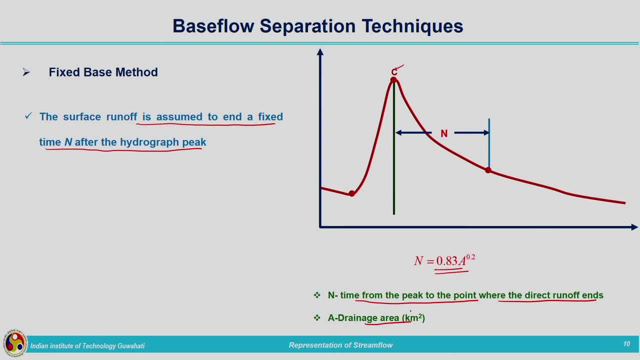 effect taken by the человека. Okay, So which not includeish? Which not includeish for the body: C, C. Yeah, The base flow before the surface runoff has begun is projected ahead to the time of the peak. 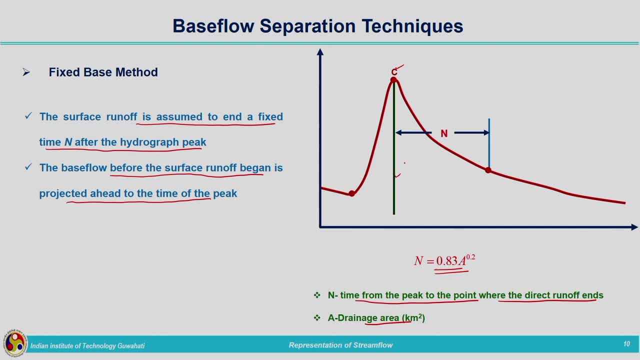 So we have dropped. a perpendicular from the peak and base flow contribution line is projected forward like this, Then we will extend. a straight line is used to connect this projection at the peak to the point on the recession limb at time n after the peak. So we have already marked that particular point n days after the peak. 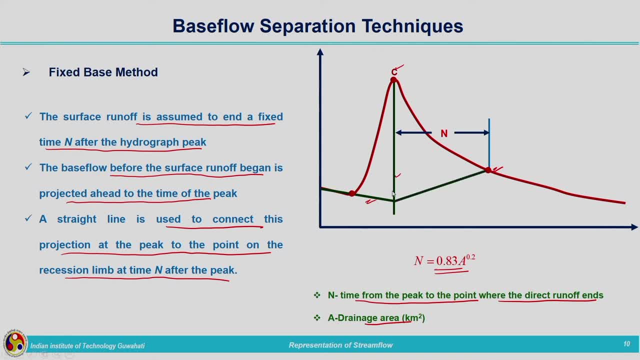 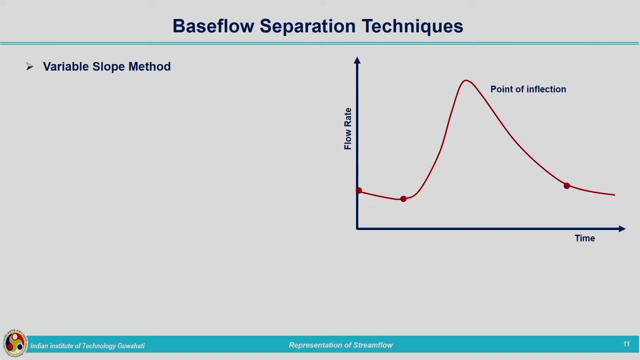 So we will be connecting this line with that particular point and below what is coming, that will be subtracted from the total stream flow So that subtracted one will be providing you the base flow. This is fixed base method and the third method is the variable slope method. 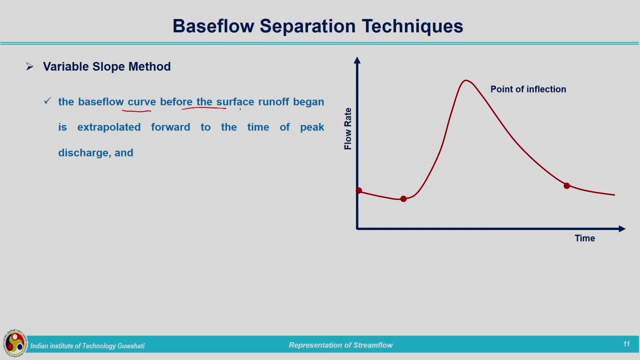 In this case the base flow curve before the surface runoff is projected ahead to the time of the peak. So we have already marked that particular point n days after the peak. So the base flow curve is projected ahead to the time of the peak. So we are checking it here and the base flow curve before surface runoff has begun is extrapolated. 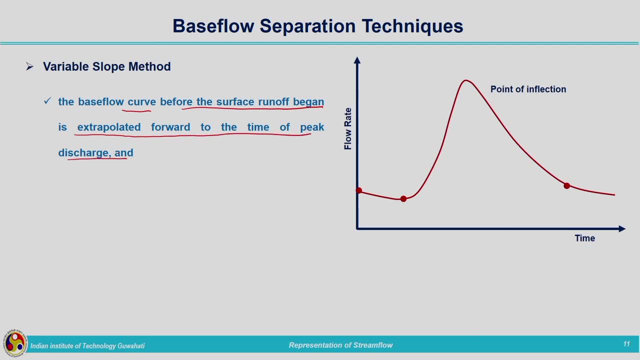 forward to the time of peak discharge. So you can see here that is our base flow region, beginning base flow region that is extended like this: It is joined with the line from the peak. and then what we are doing: the base flow curve after surface runoff has ceased is extrapolated backward to the time of the point of inflection. 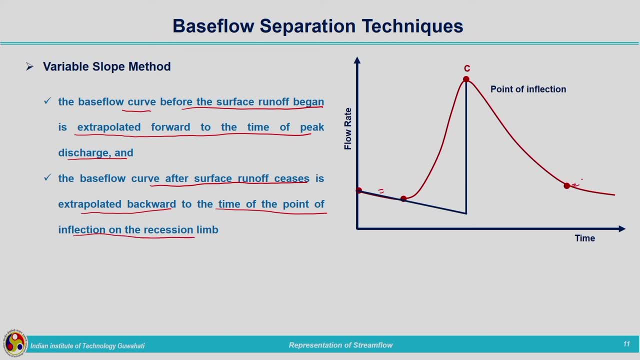 the recession limb here. this is the point where the base contribution from runoff stops. so from that particular point we will interpolate from there. the base flow contribution only will be shown after that. that base flow contribution after the recession limb will be extrapolated backwards this way. then from the point of inflection we will be dropping the perpendicular. 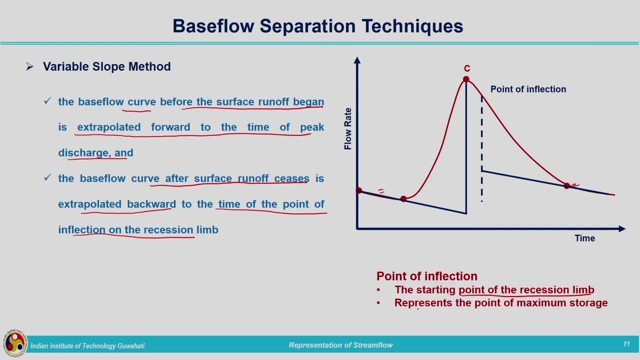 that is point of inflection, is the starting point of the recession limb and it represents the point of maximum storage. after that, what we will be doing: the end points of the extrapolated curves are connected by means of a straight line. this way, we will be connecting and beneath the 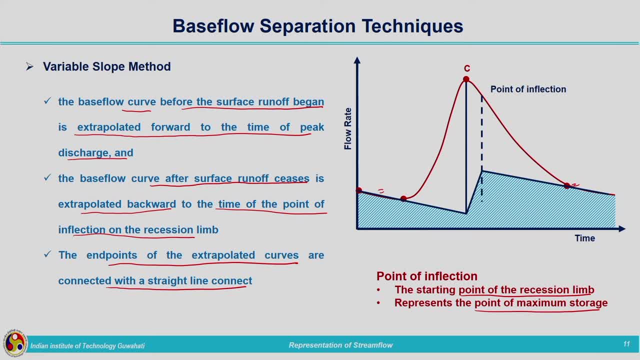 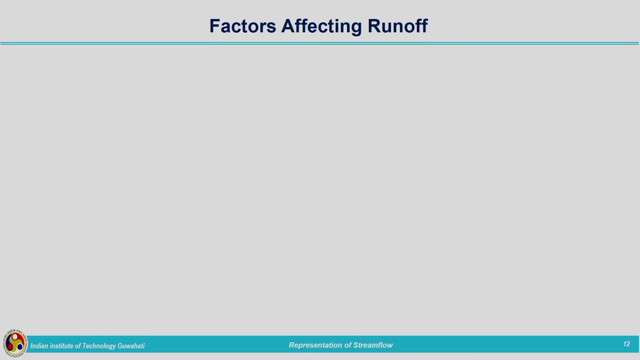 these lines, the extrapolated lines, whatever, marked by that blue lines will be hatched and that is representing our base flow that needs to be deducted from the total stream flow to get the direct runoff. now let us see different factors affecting runoff. when we talk about runoff or the stream flow, which are the different factors influencing? 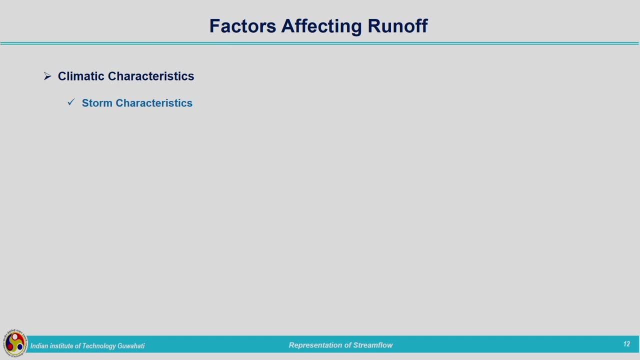 first one is the climatic characteristics. it includes the storm characteristics, initial abstraction and also evapotranspiration. then second one is classified as physiographic factors. in physiographic factors it includes the total stream flow to get the direct runoff and theジャーツということ includes the catchment characteristics and infiltration. 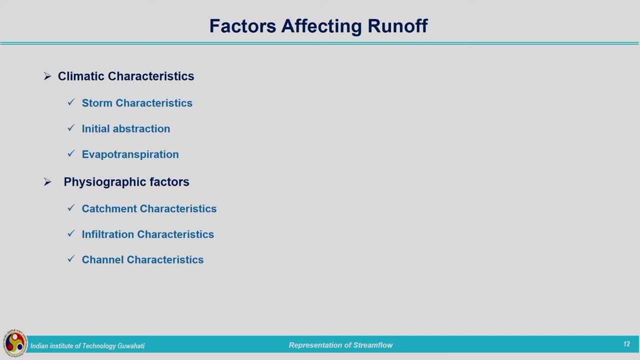 characteristics, also channel characteristics. so factors which are affecting render includes climatic characteristics and also physiographic characteristics. climatic characteristics includes the storm characteristics, initial abstraction and evapotranspiration, and physiographic factors involves the catchment characteristics, infiltration characteristics and channel characteristics. Coming to catchment characteristics, it includes the shape, size and slope, drainage density. 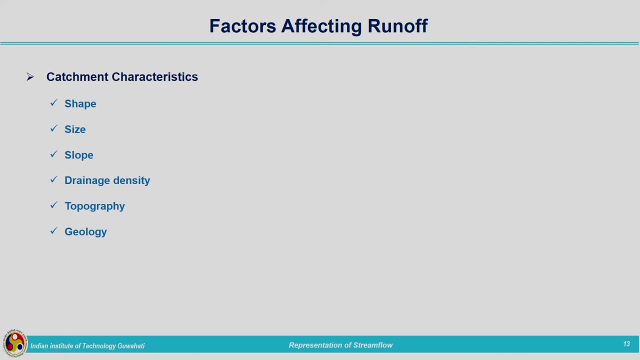 topography and geology. Definitely, depending on the catchment characteristics, the contribution of water towards the drainage basin outlet will be different. If it is a steep catchment or the slope is more, the water reaching at the outlet will be at a faster rate compared to a flat terrain. 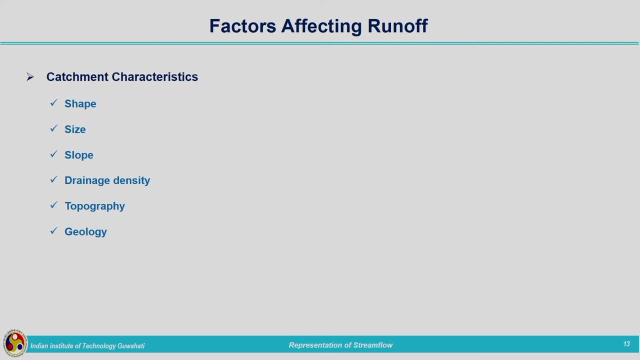 So shape, size and slope, and also drainage density. If more drainage density, faster the rate at which the water will be reached at the outlet point, And topography, geology, all these matters. all this affects the stream flow, which is 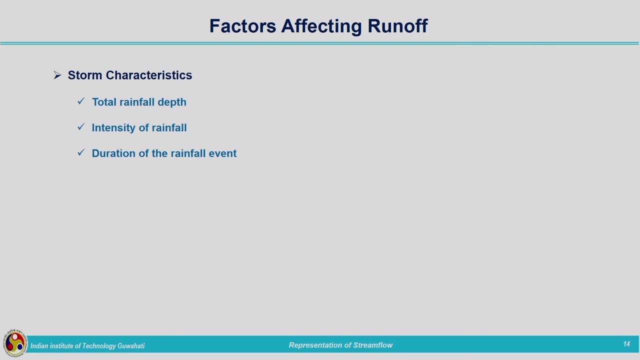 measured at the outlet point And when coming to storm characteristic. it includes the total rainfall depth, the speed, intensity of rainfall, duration of the rainfall event. If it is for a very short duration, maybe entire water may be lost. as initial abstraction, It will not be contributing anything towards. 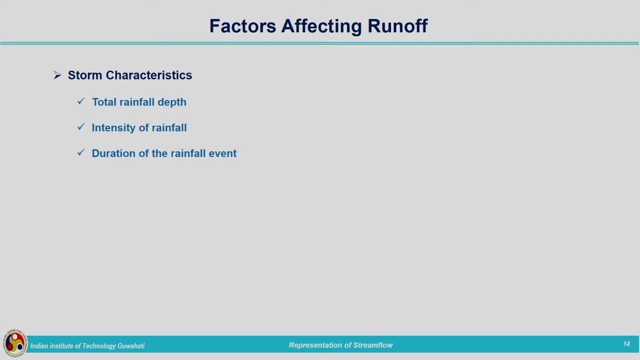 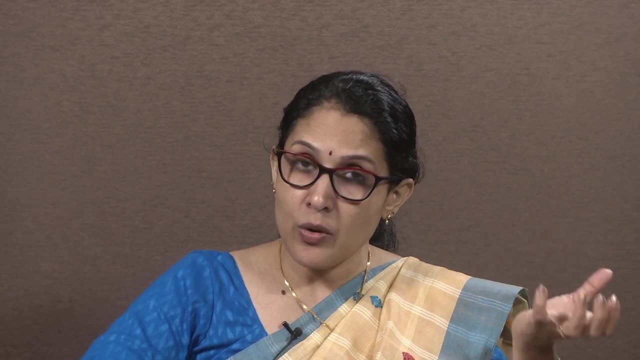 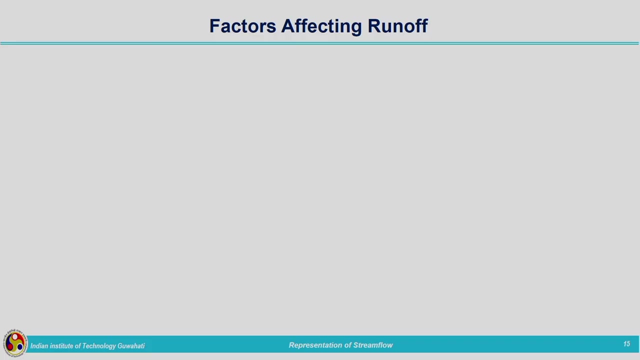 the runoff component and if the storm is lasting for a long time, duration is very high. in such cases, even after satisfying the storage components, runoff will be starting and it will be contributing towards the stream flow. Now, different factors affecting runoff, that is, we were discussing about catchment characteristics in detail. we can see: 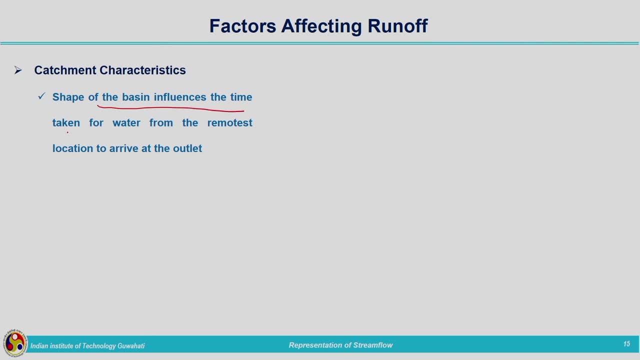 The shape of the basin influences the time taken for water from the remotest location to arrive at the outlet. That we have seen the time taken by water to travel from the remotest point to the outlet point. This is termed as the time of concentration. So, depending upon the shape of the basin, the 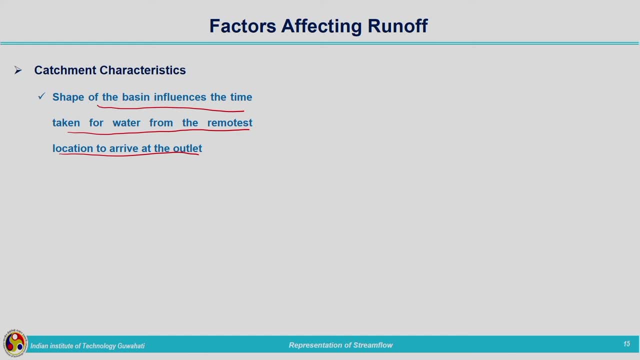 time or the time of concentration will be different, So that matters. how much is the runoff value? it depends upon time of concentration. So if the watershed is like having this shape, which is having stream networks like this, it is termed as fan shaped watershed, and you 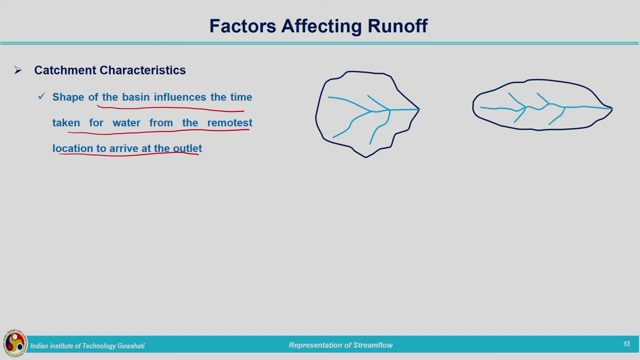 can calculate the time of concentration. So if the watershed is like having this shape, which is having stream networks like this, it is termed as fan shaped watershed and you can calculate the time of concentration. Compare it with an elongated watershed. it is a very lengthy watershed In both the cases when you 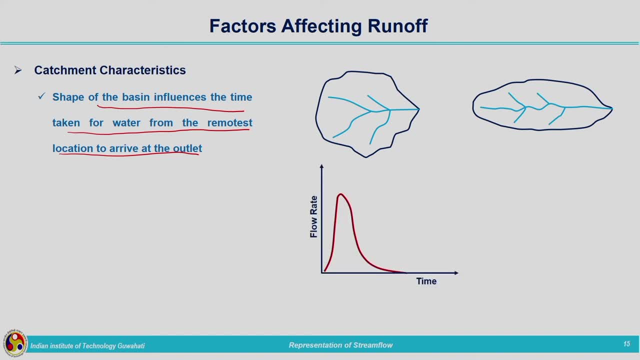 see if you plot the storm hydrograph. in the case of fan shaped watershed, we are getting a hydrograph like this which is having a peak coming fast, And in the case of elongated watershed, you are having a flat peak That is the entire water. 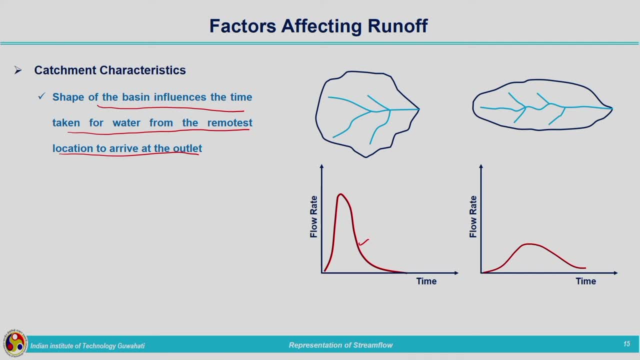 is contributing and the peak is attaining for a long time. Gradually the peak is attaining but in the case of first one fan shaped with more drainage density, very good drainage system is available for the flow to take place. In that case peak will be attained faster rate compared. 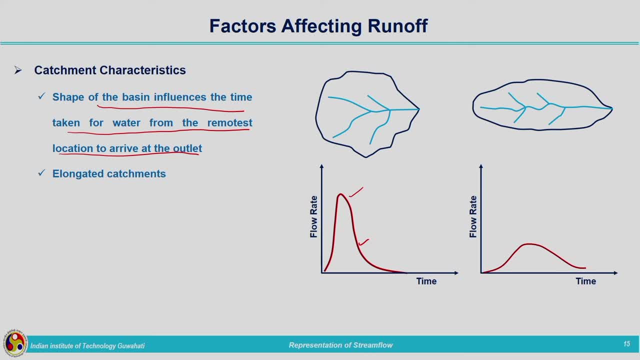 to the other one Elongated catchments as lesser peak compared to fan shaped catchment of the same area and longer runoff durations than a fan shaped catchment. So you can compare the hydrographs. in both the cases One is having a sharp peak and in the other case it is having a flat peak. 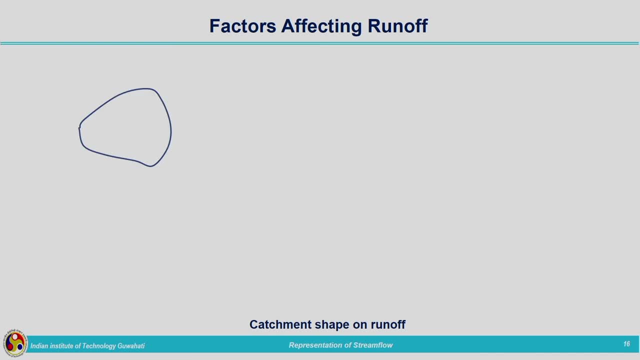 Now coming to catchment shape on runoff Differential between the two cases, Different catchments we can consider Here. in this case we are having the catchment wider, near to the outlet point. Our outlet point is here and stream is starting from the furthest point and 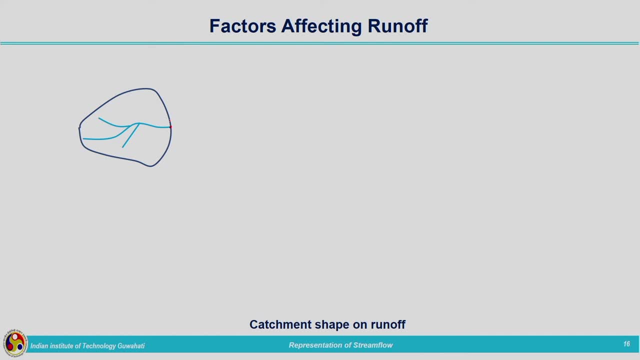 away from the outlet point, the watershed is reduced in width. Second, one is, on the other hand, at the outlet point. the width is less. It is becoming wider as the distance from the outlet point. Then, third, one is having a shape as shown in this, So streams are present in the watershed, like this: 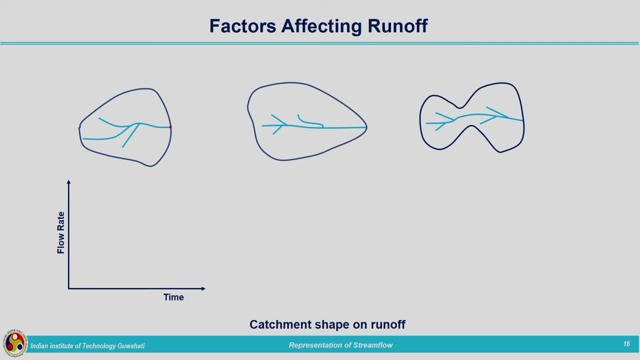 and we can plot the corresponding hydrographs from all these watersheds. In this case you can see the peak at this point as attained at a faster rate and it is skewed towards the left. So peak has attained early and after that also contribution of flow coming from the farthest point. 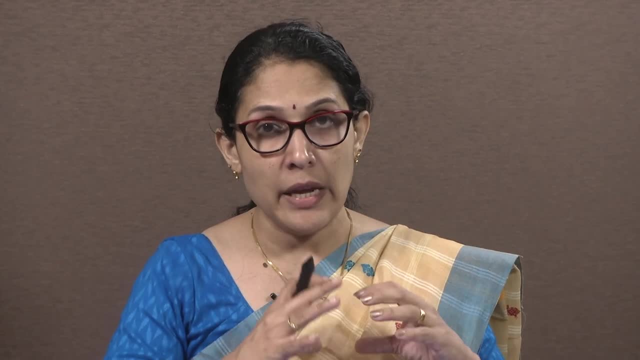 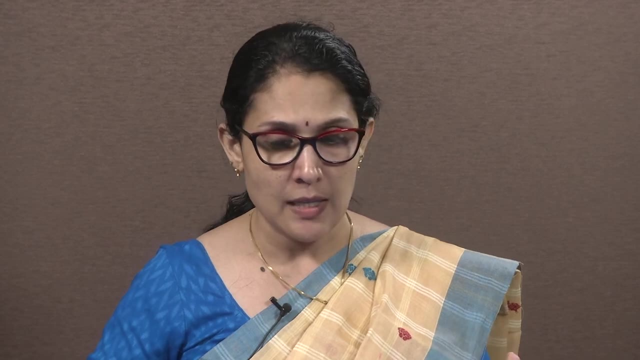 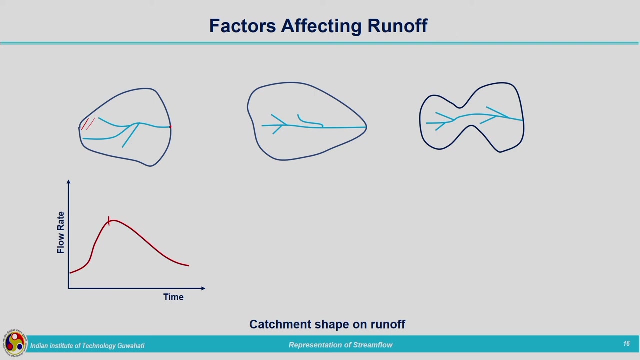 But the peak is due to the major area that is very close to the outlet point. That is why we are having a skewed peak in the first case. Second case: you can imagine how it will be: Maximum area is far away from the outlet point, So definitely we will be having a skewed peak towards the right. 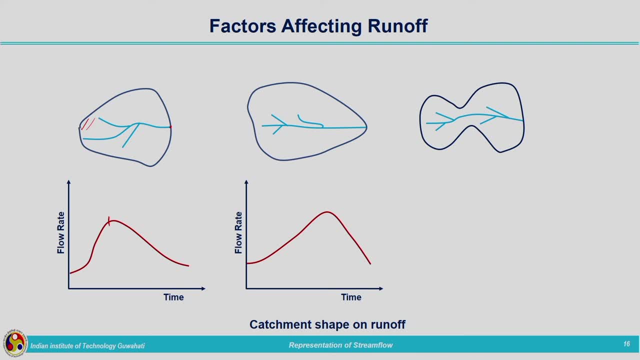 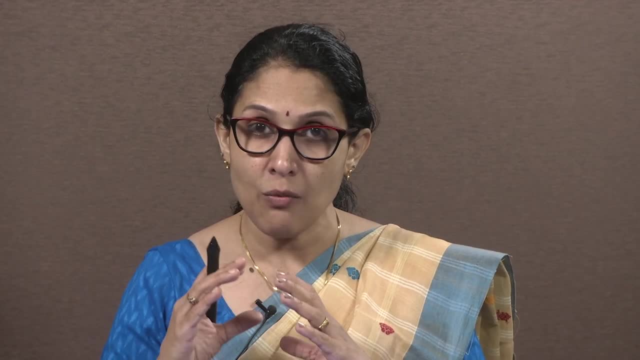 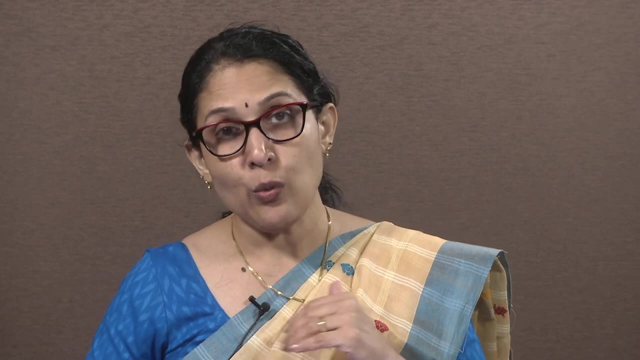 So it will be like this: Initially, the runoff which is reaching at the outlet point will be less, and after certain time, only entire catchment will be contributing water to the outlet point. That is why the peak will be skewed towards the right hand side. Now, in this case, third one, how it will be. 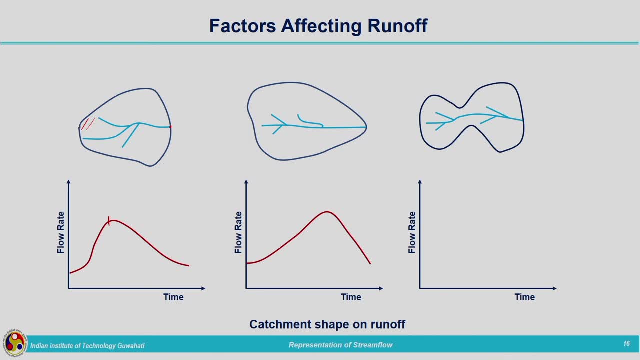 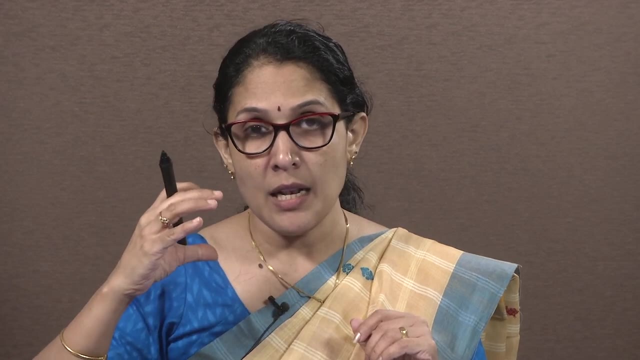 In the case of third one, you can understand that we are having maximum area here and also we are having large area compared to the central portion. So in this case the hydrograph will be having multiple peaks. That is initially initial area contribution will be high Then because of the 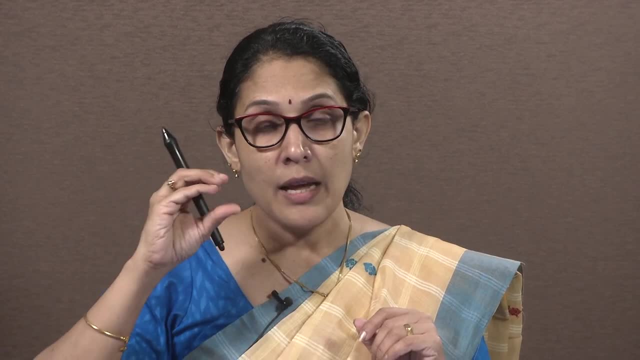 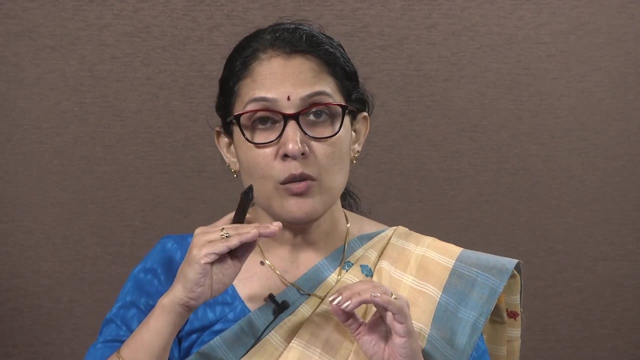 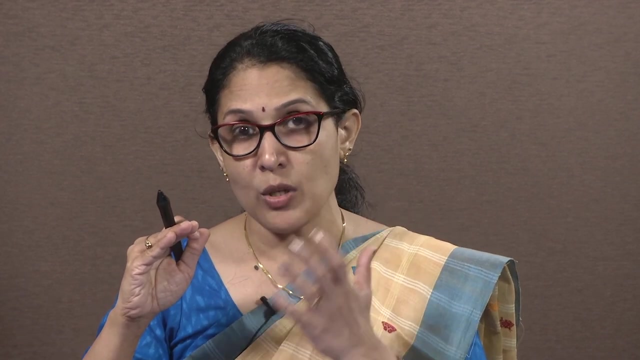 reduction in area. the contribution is reduced Again the farthest points. farthest area is more compared to in between area. So initially the flow will be rising, then reducing, then when the entire catchment starts contribution at the outlet point it will be increasing. So these are the 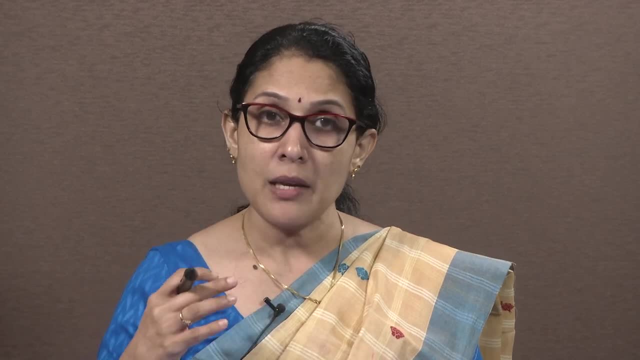 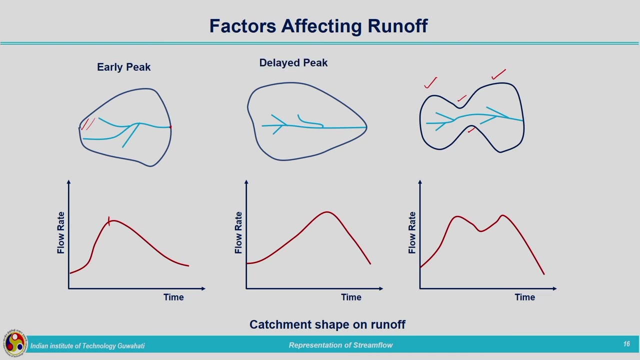 different types of hydrograph which we can experience from different shapes of watersheds. In the first case, we are having early peak. Second case, delayed peak and in the third case, we are having multiple peaks. Now, very important thing which you need to understand: what is the? 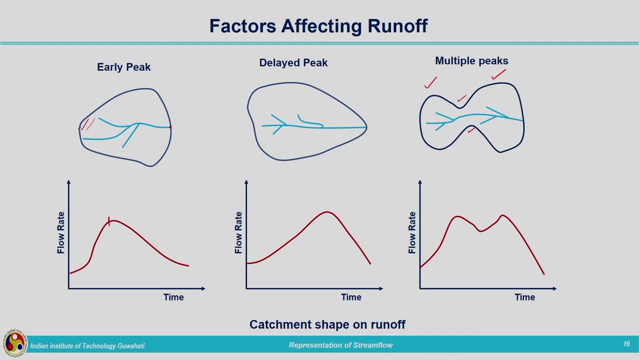 influence of urbanization on the environment. What is the influence of urbanization on the environment? What is the influence of urbanization on the environment? What is the influence of urbanization on the hydrograph? So the effects of urbanization on the flood hydrograph include increased total. 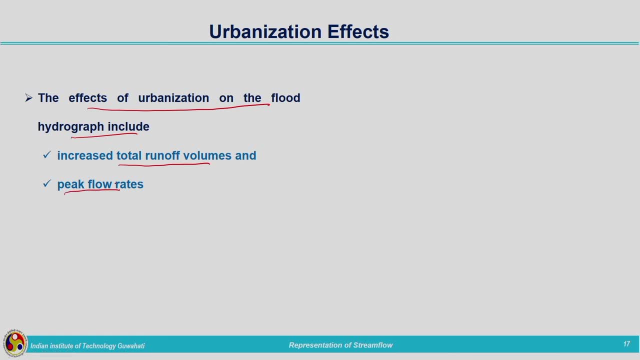 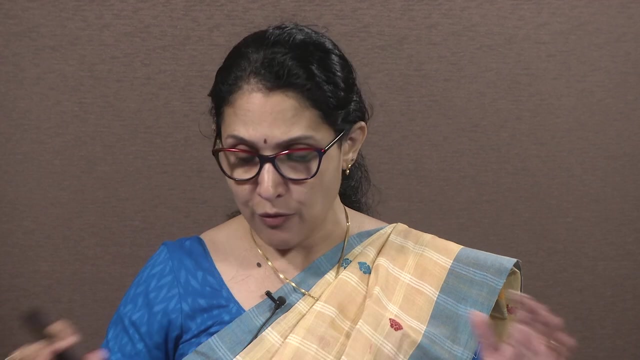 runoff volume, then peak flow rates. We can see by means of a graph flow rate along the y-axis and time along the x-axis. This is the one which is having a flat peak and the time taken for the runoff is very large. So you can understand. 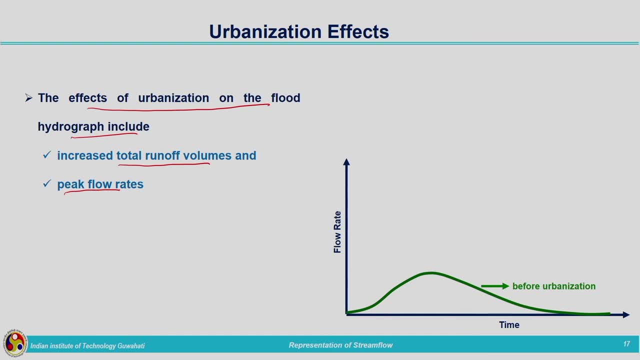 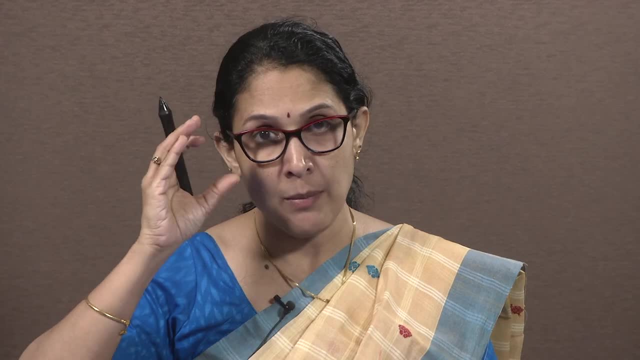 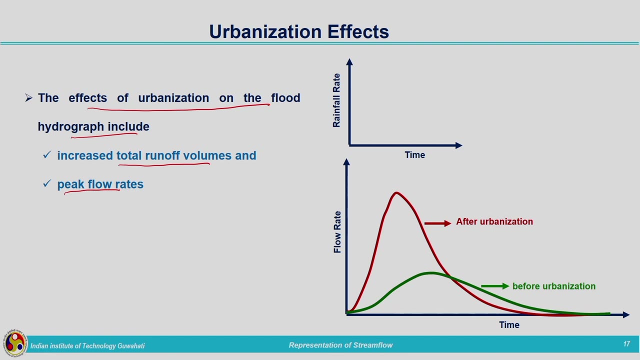 that this is before urbanization and in the case of after urbanization, peak will be very high and time taken to peak to attain will be less. This is after urbanization. Now, when we are plotting the rainfall rate versus time, if this is a uniform rainfall we have, 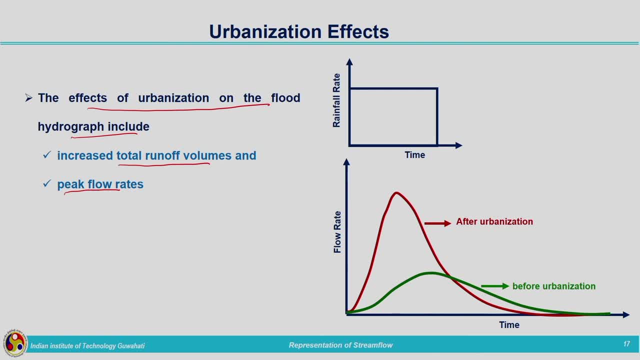 considered rainfall intensity. we have considered out of that total rainfall. this green line is representing the infiltration before urbanization. In the case of before urbanization, impervious areas will be less, So we will be having more and more infiltration taking place. So that is. 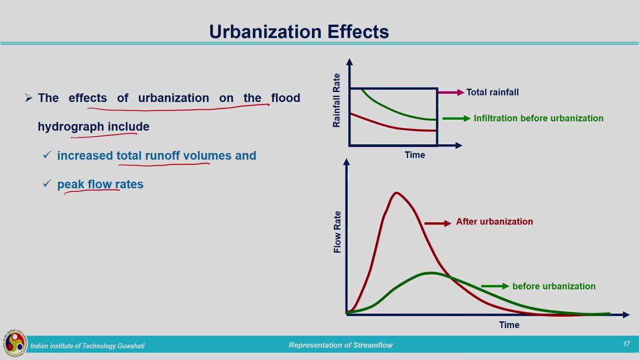 represented by this green curve. and in the case of after urbanization, what will happen? impervious areas are increased. due to that, the water which is infiltrating into the ground gets reduced. Because of that, the runoff volume will be increasing. So this much amount of extra water is contributing towards runoff because of 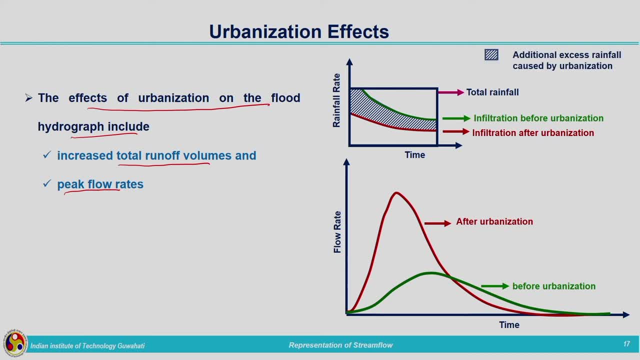 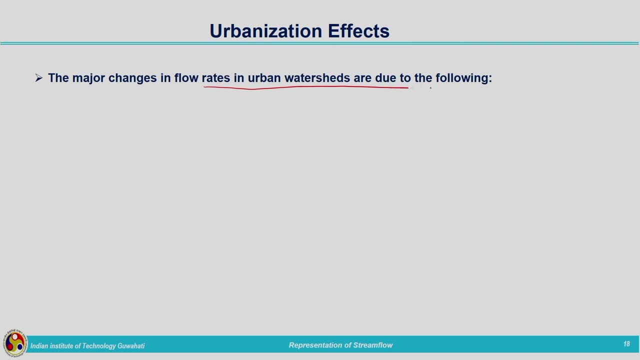 urbanization. Additional excess rainfall caused by urbanization is marked by this hatched area. Now, major changes in flow rates in urban watersheds are due to the following reasons. That is, the volume of water available for runoff increased because of the reduction in the amount. 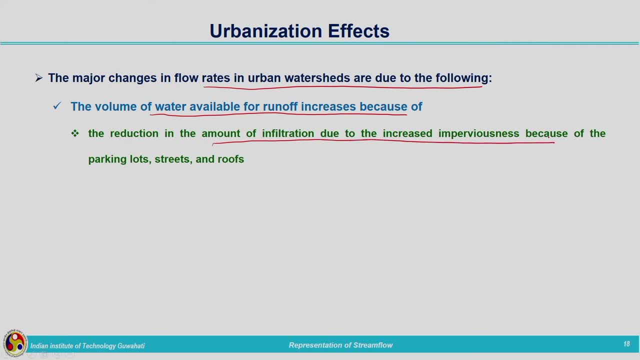 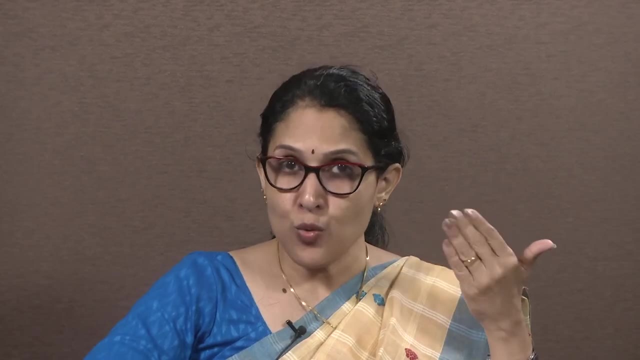 of infiltration due to the increased imperviousness because of the parking loads, streets and roofs. In the case of urbanized area, paved areas are more. Because of the paved characteristics, water infiltrating will be less. We have seen two types of hydrographs: annual hydrographs and also storm hydrographs, So different components of